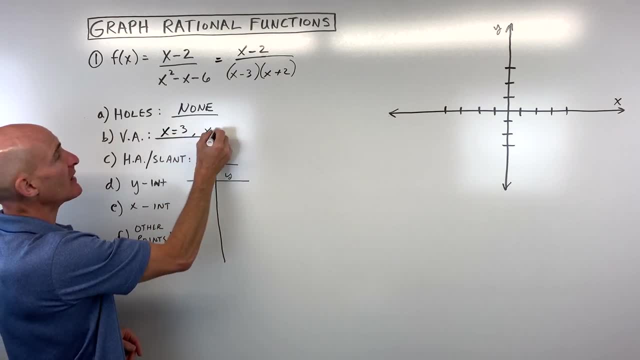 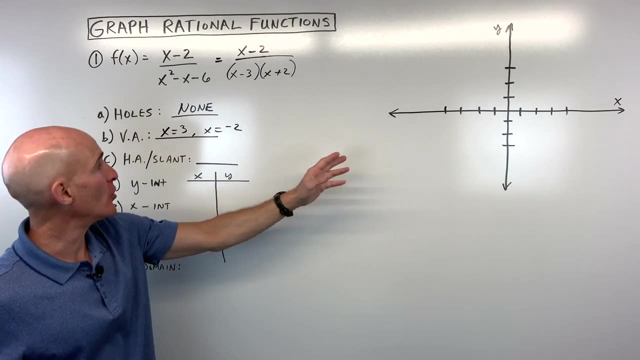 vertical asymptotes at x equals 3 and x equals negative 2.. Now what I like to do is, as I figure things out over here, I like to kind of graph it as I go. So x equals 3 is a vertical line right here. 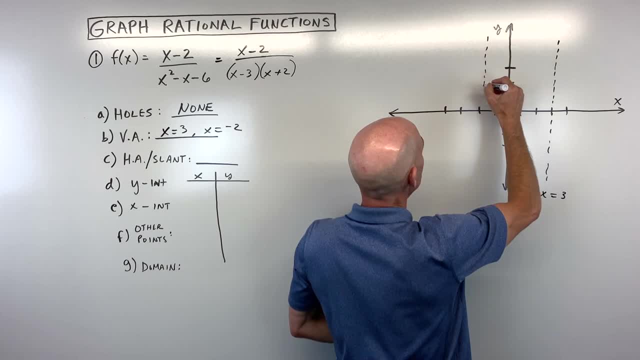 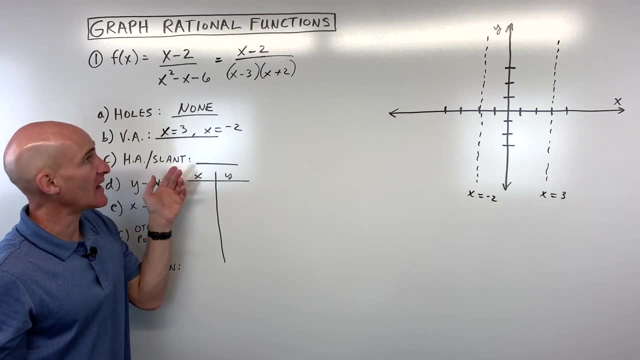 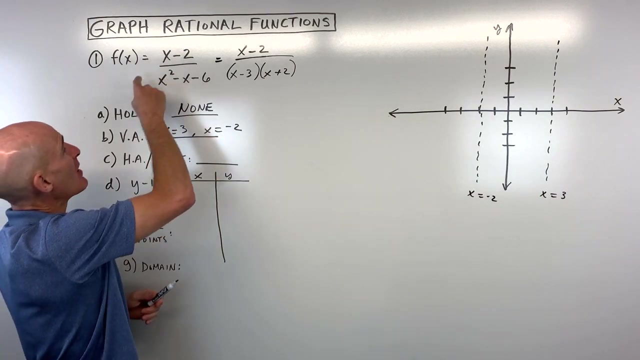 And x equals negative. 2 is also a vertical line going through negative 2.. Okay, so now let's talk about the horizontal asymptotes or the slant asymptotes. So when you're analyzing whether it has a horizontal or a slant, you look at the highest power term in the numerator and the highest. 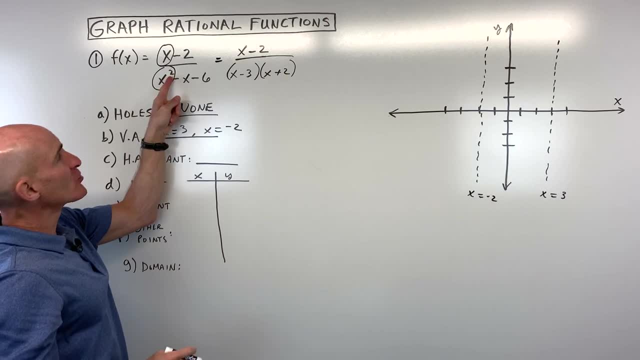 power term in the denominator. Now, if the denominator's degree is higher than the numerator's degree, then the horizontal asymptote is going to be the line: y equals zero. okay, and the way to understand that is: imagine, as x gets larger and larger, like if i put in 1 for x, 100 squared is ten thousand. 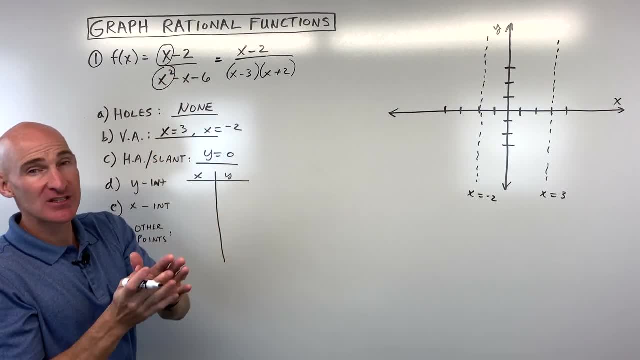 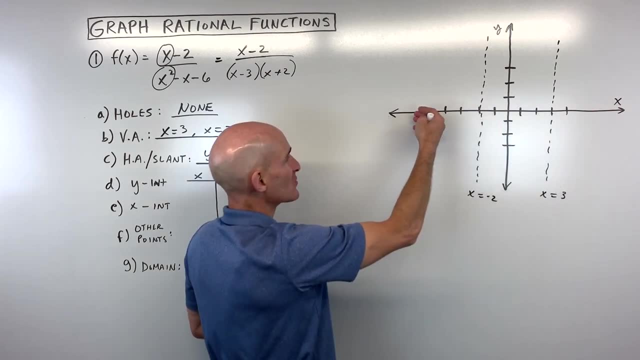 and this is one hundred 100 divided by 10 000. that's going to be a very small number. it's getting closer and closer to 0. so what that means is, as x gets large and larger as you go to the right, Whereas x goes to, let's say, negative infinity, you go to the left, this whole fraction is: 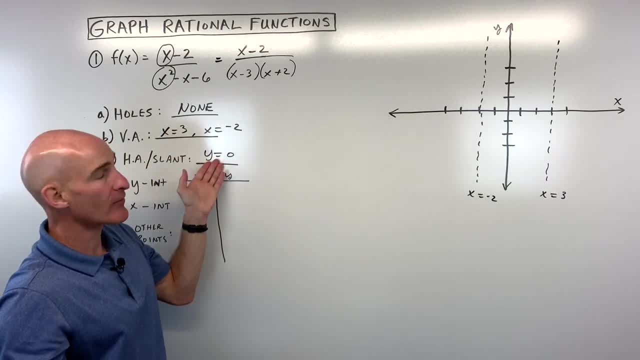 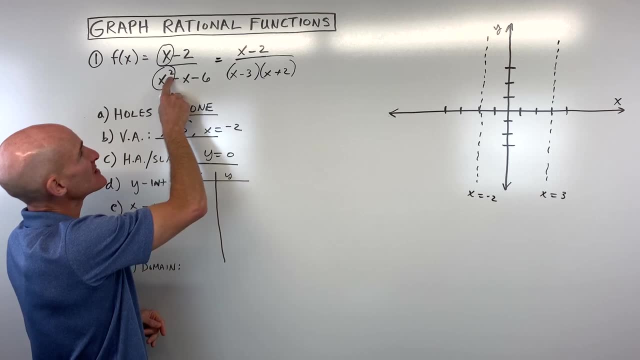 going to get smaller and smaller. It's going to go to zero, And so that's why we have our horizontal asymptote: of y equals zero. Now you might be saying, Mario, what about these other terms here? Well, you can see, this x squared is growing faster than this x. 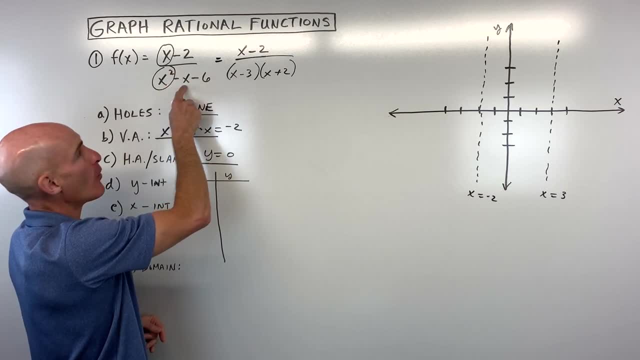 So as x gets bigger and bigger, this term is going to basically outpace these guys here. Same thing in the numerator. This is going to be growing much faster than minus two. So as x gets really big, this kind of acts more like x over x squared. 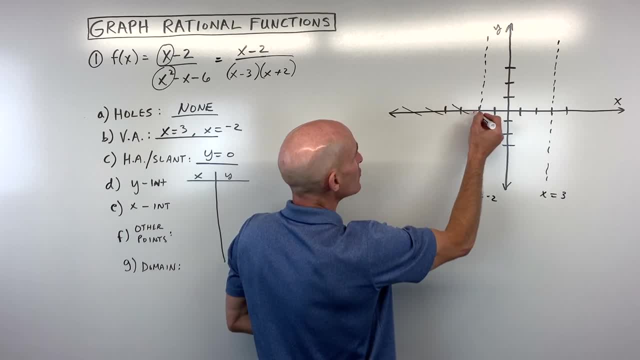 And that's how we're getting that horizontal asymptote here, which in this case is right at the x-axis. I kind of like to put the asymptote kind of like on a little bit of a diagonal like that, just so that I can see it. 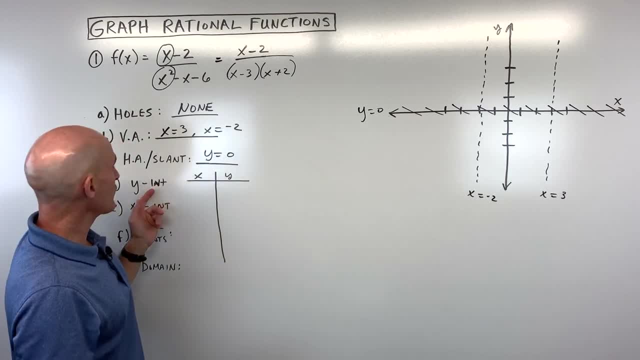 It doesn't blend in with the x-axis. Okay, now for the y-intercept. So y-intercept means where does it cross the y-axis? Well, that's going to occur when x is equal to zero. okay, Because when x is zero, we're not going to get zero. 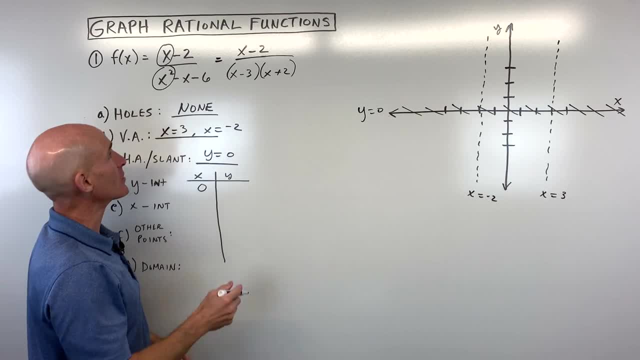 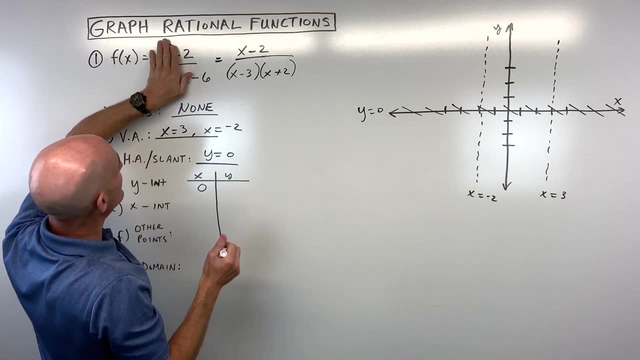 We're going left to right. You're just along this vertical y-axis here. So if I put zero in for x, that's going to cancel out this term, this term and this term. So anything that has an x in it, those guys are going to cancel out. 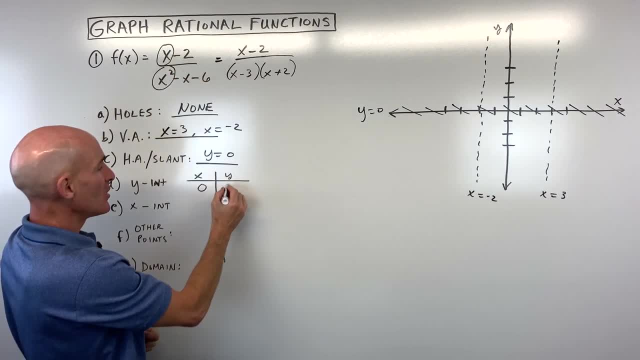 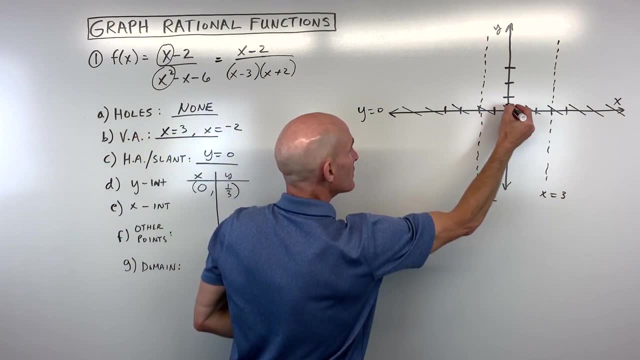 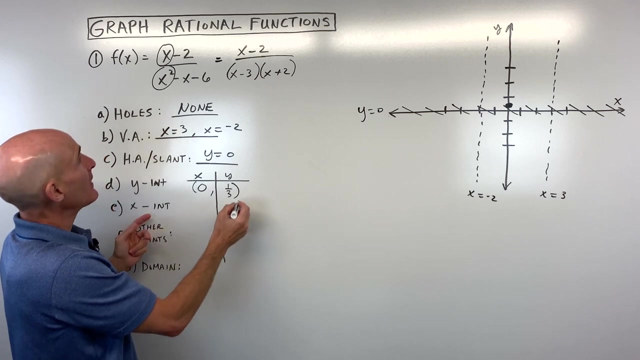 And you can see we have negative two divided by negative six, which is one-third. So there is our y-intercept: zero comma one-third, which is right about here. Now for our x-intercept, we do the opposite. We set y equal to zero. 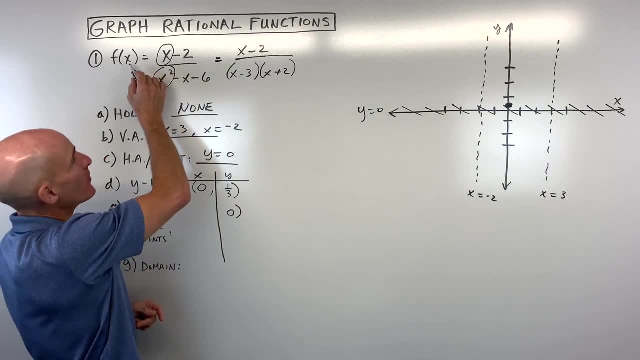 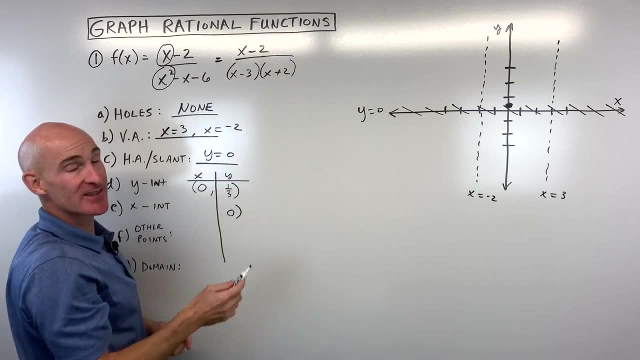 And in order for f of x or y to be equal to zero, the only way this is going to be zero is if the numerator is zero. right, Because if you have a fraction, the numerator is zero and the denominator is not zero. that. 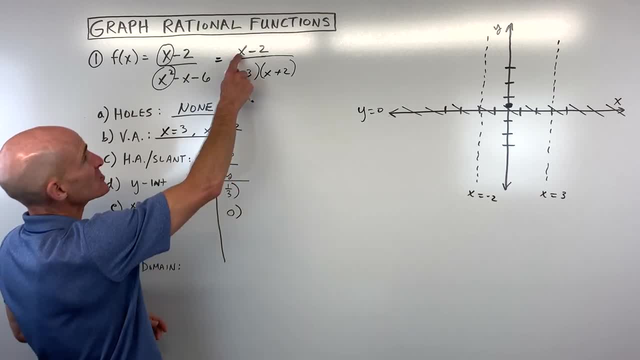 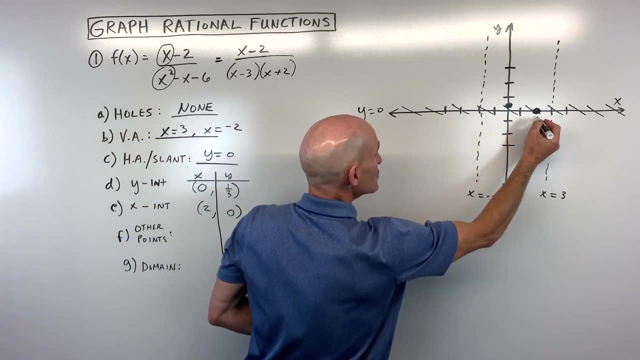 whole fraction is going to be equal to zero. So a shortcut is just to set the numerator's factors to zero, and that's going to give you two. So in this case we have an x-intercept of two right here. Now, for some students that might seem a little bit confusing. 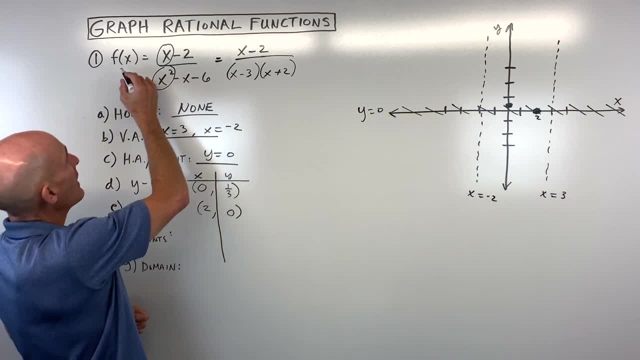 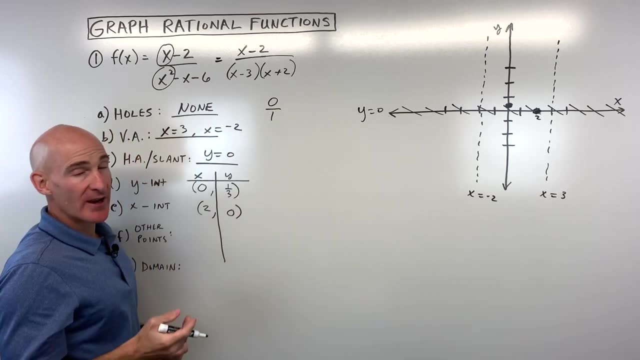 So what you might want to do is, you might want to do this. You might want to say: well, Mario said, set y to zero, So that's going to be: f of x is equal to zero. Zero is like zero over one right. 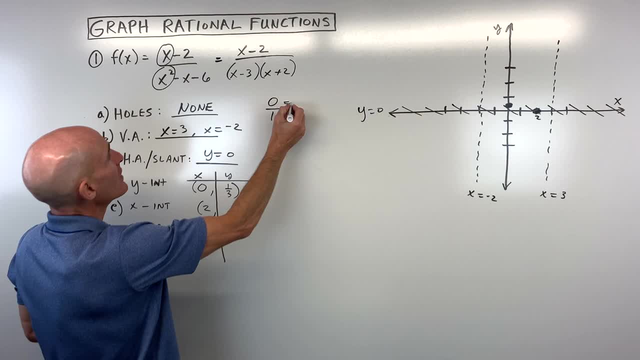 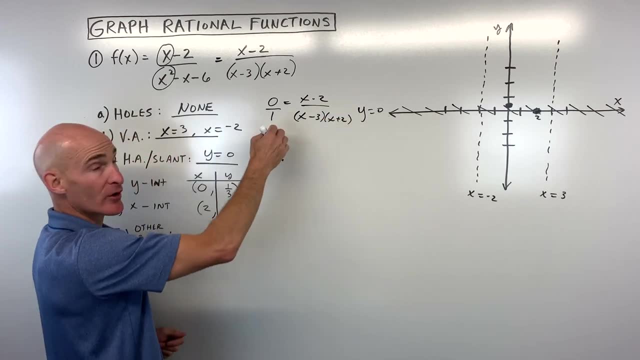 Because anything divided by one is itself. that's still going to be zero. And then over here we have x minus two over x minus three times x plus two. Now you know the cross product where you multiply on the diagonals. So zero times this quantity gives us zero. 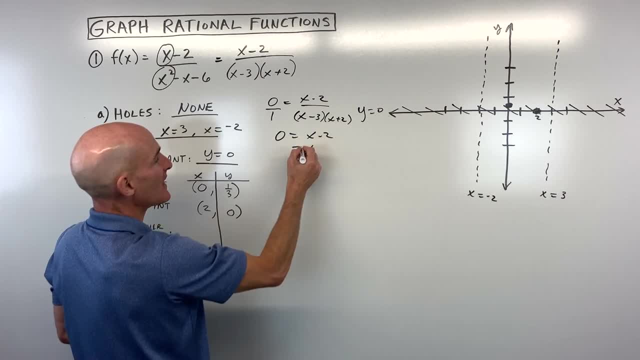 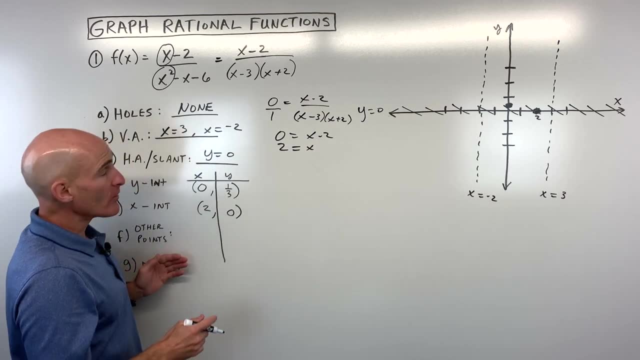 And x minus two times one is itself, And then if we add two to both sides, you can see we're getting x equals two. That's another way to do it. It's just to do that cross product. Okay, now we've got some pretty good framework here. 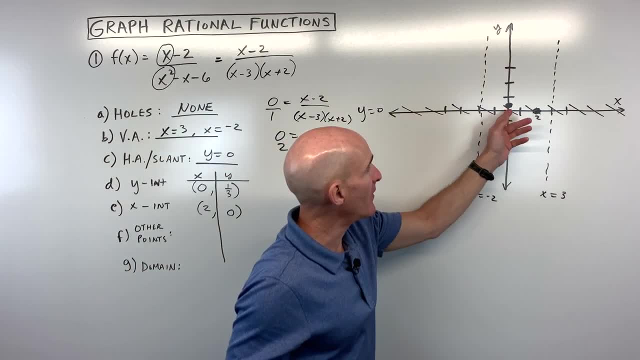 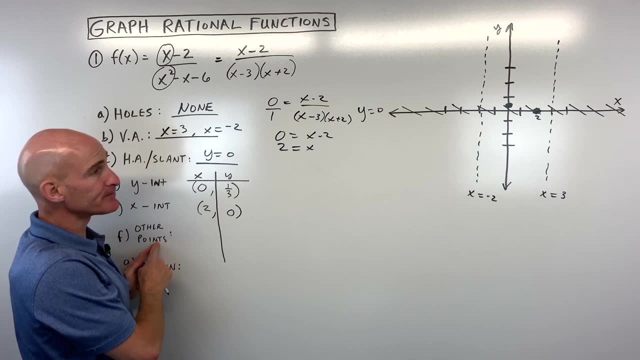 We have our vertical asymptotes, We have our horizontal asymptote, We have our intercepts. The thing to focus on now are some additional points to help us to get a good graph here. Now, what's interesting is: you can cross a horizontal asymptote, but you cannot cross. 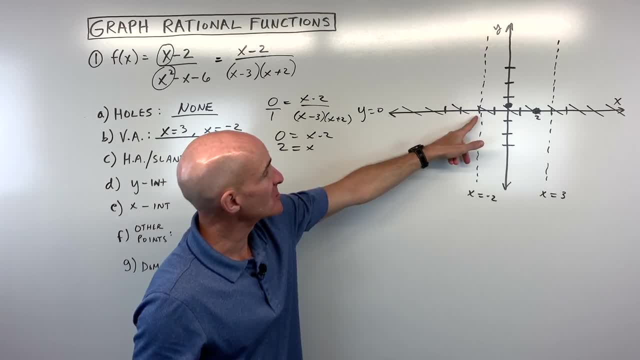 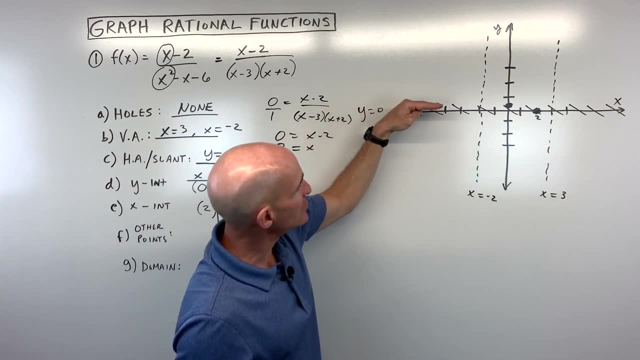 a vertical asymptote, And the reason is is because if x was negative two- we talked about this earlier- you'd be dividing by zero. It's undefined. Same thing over here with three. So what happens is, when you approach a vertical asymptote, it's like a brick wall. 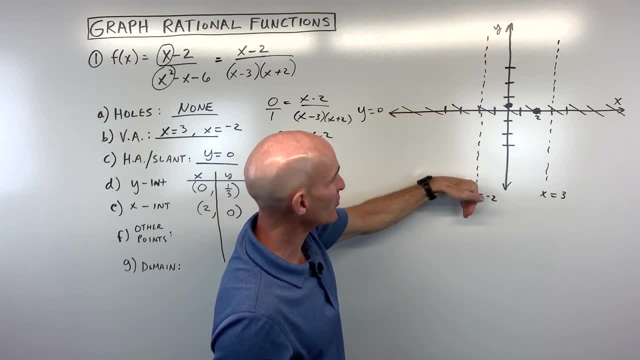 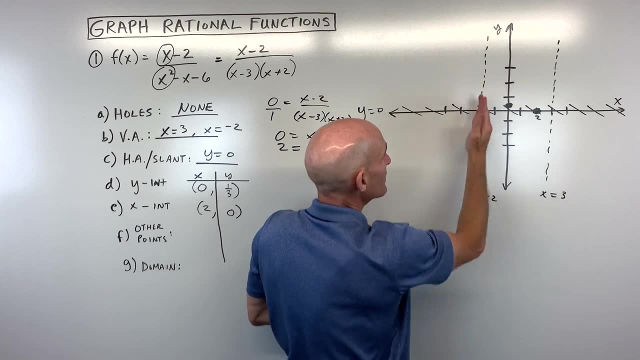 You either have to turn up towards positive infinity or down towards negative infinity. You can't go through that vertical asymptote. So what I like to do is I like to pick some points on either side of the vertical asymptotes, And what we're going to do is what's called sign analysis. 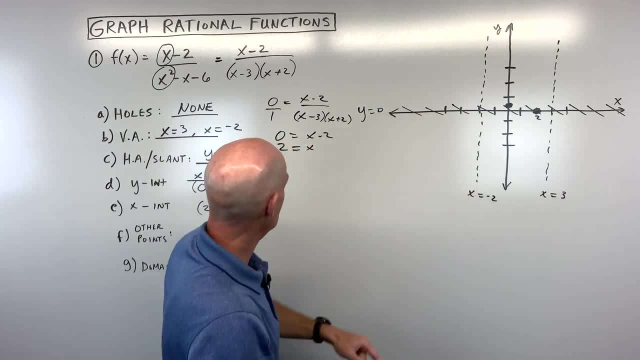 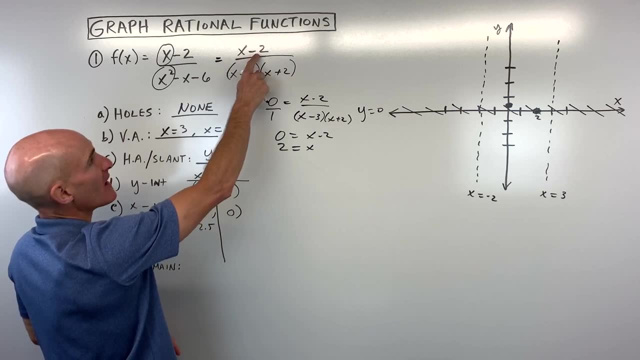 So, for example, if I pick like a negative 2.5, okay, let's just put this in our table here: Negative 2.5.. Okay, I'm going to write it in this factored form right here. So negative 2.5 minus 2 is negative 4.5, but I'm just going to write it as a negative. 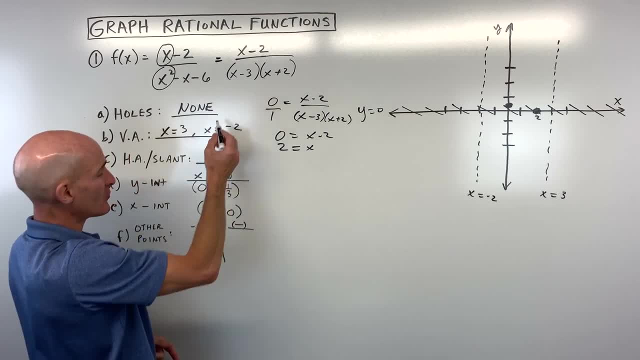 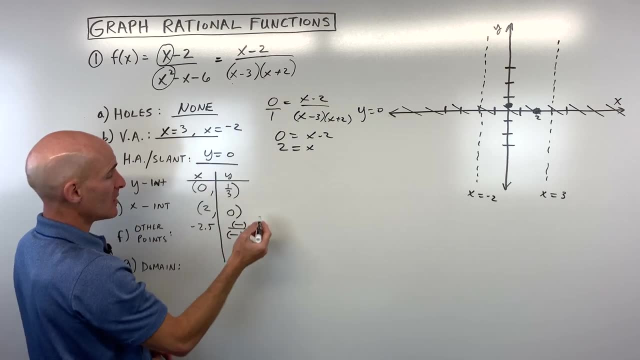 Okay, I'm not going to focus on the number. I'm just going to focus on whether it's negative or positive. Negative: 2.5 minus 3 is negative 5.5. That's negative. Negative 2.5 times or plus 2 is a negative 0.5.. 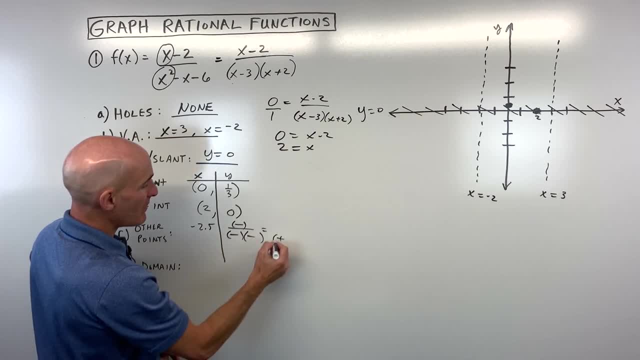 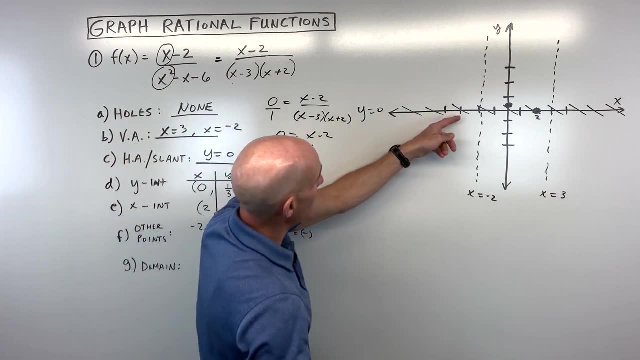 That's negative. And notice what we have here: A negative times a negative is a positive. A negative divided by a positive is a negative. So what that tells me is that Negative 2.5, this graph is going down towards negative infinity. 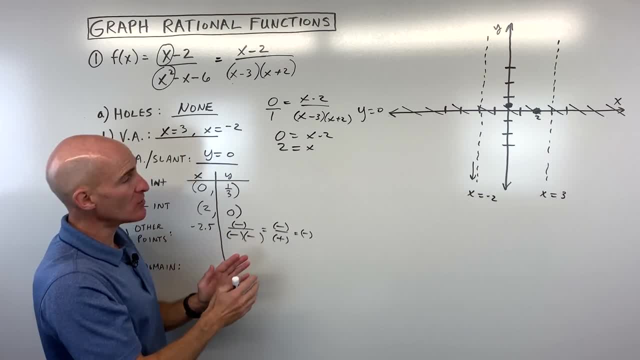 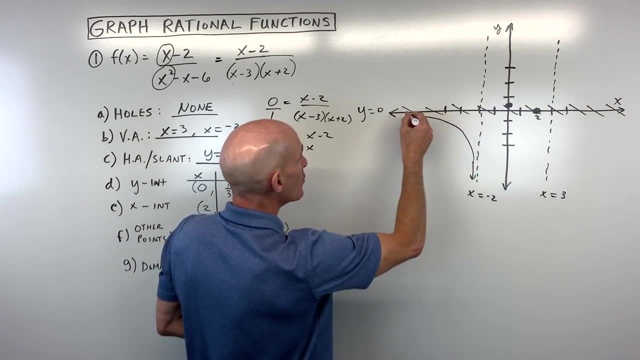 Now, if you want to get an actual number, go ahead, You can certainly do that. But the main thing is it's going down as you get closer to this vertical asymptote And when you go this direction, you're approaching this horizontal asymptote at y equals 0.. 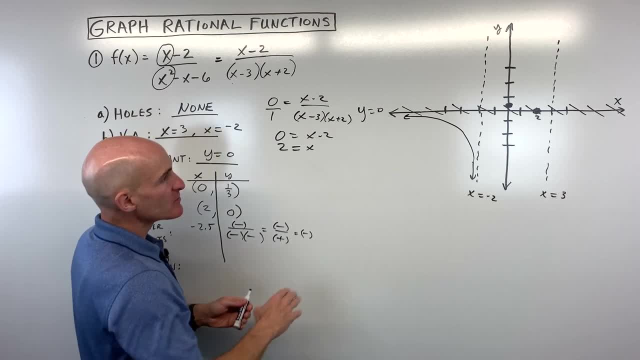 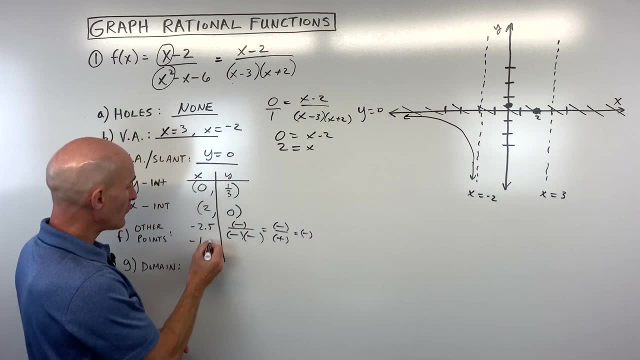 So you can see here we're getting this branch of the graph. Now let's pick a point on this side of the vertical asymptote. Maybe let's do negative 1.5.. So if we plug in negative 1.5. We get a negative 3.5, a negative 4.5, and a positive 0.5.. 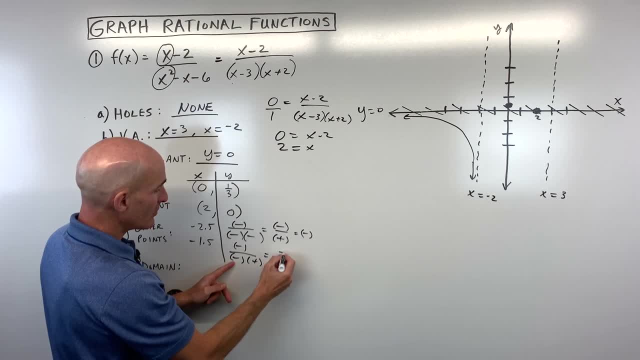 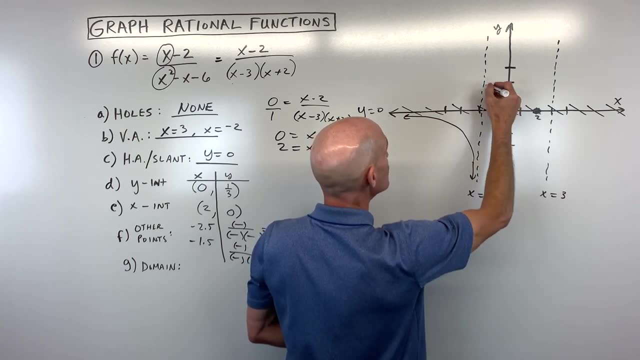 So now look what we have. We have a negative times a positive, which is a negative in the denominator Negative divided by a negative is a positive. That tells us when we're approaching this asymptote from this side. it's going up towards. 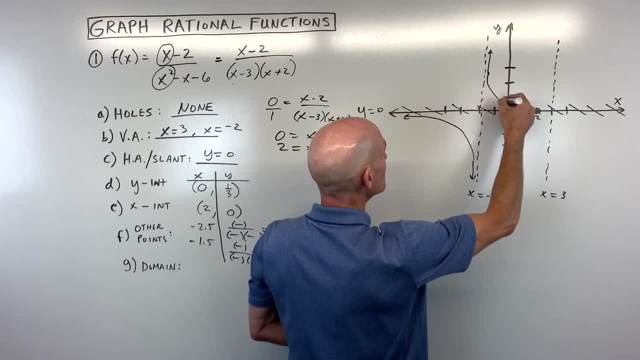 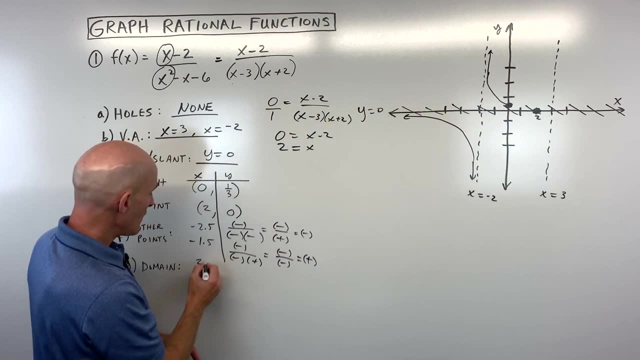 positive infinity. So here you can see the graph's kind of looking like this. right Now let's pick a point on this side of the vertical asymptote, Maybe 2.5. So if we plug in 2.5, let's say we get a 0.5, which is positive. 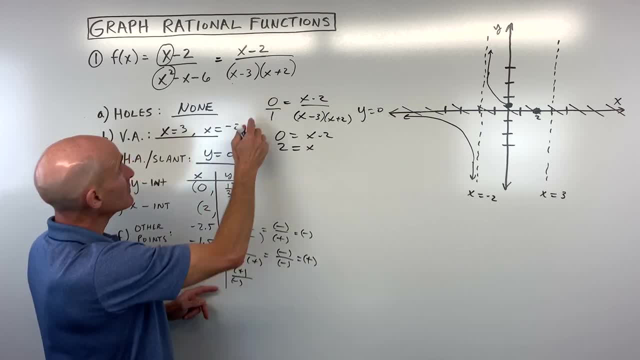 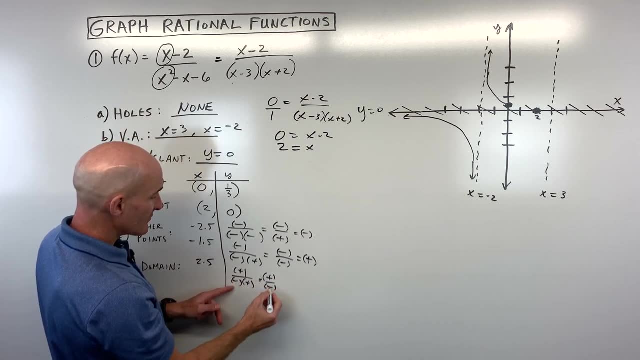 2.5 minus 3 is going to be a negative. 2.5 plus 2 is a positive And you can see a negative times a positive is a negative And a positive divided by a negative is a negative, And that tells us this is going down towards negative infinity. 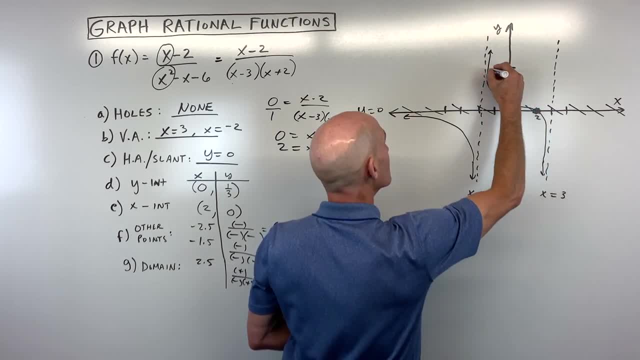 So you can see, this branch of the graph looks something like that: And then over here, let's pick maybe a negative. And then over here let's pick maybe a positive. And then over here, let's pick maybe a negative. And then over here let's pick maybe a positive. 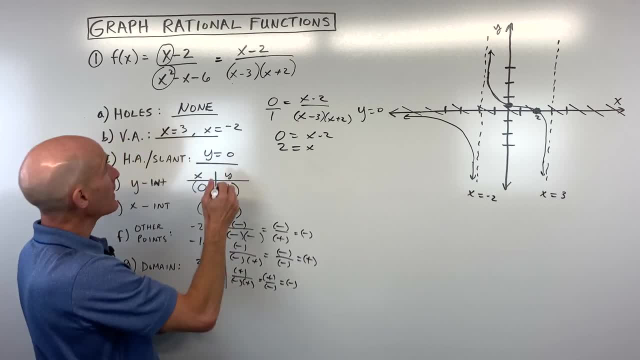 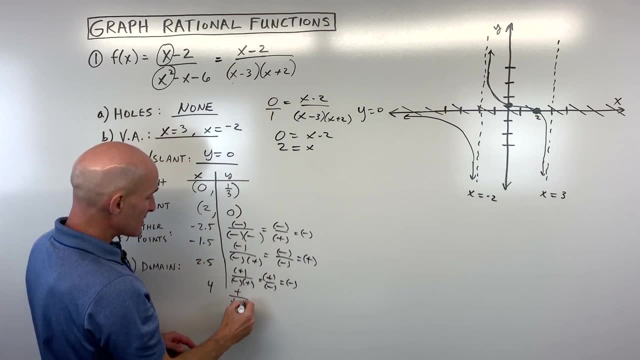 And then over here let's pick maybe a 4.. An easy one. So if we plug in 4, what do we get? We get positive in the numerator. 4 minus 3 is positive, 4 plus 2 is positive. 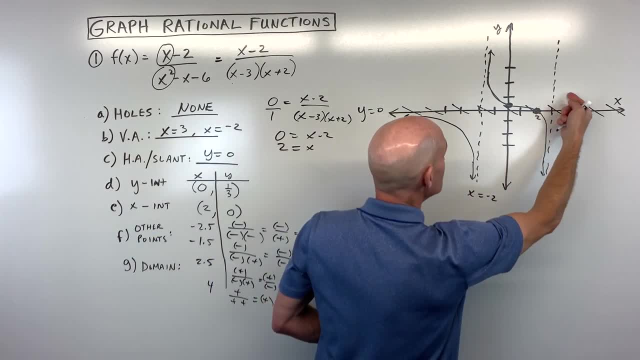 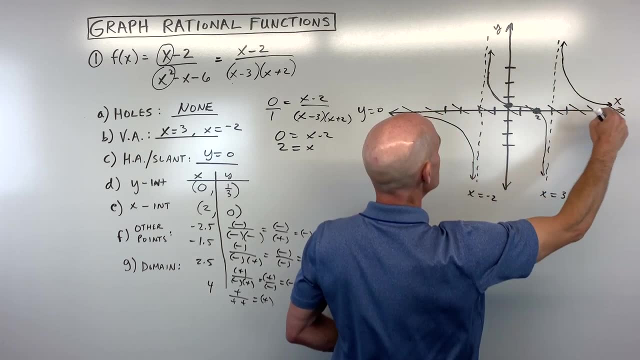 So we're getting a positive divided by a positive, which is a positive That tells us this is going up towards positive infinity. and then it's approaching the horizontal asymptote as x gets larger and larger. So you can see, we have a pretty good sketch of our graph. 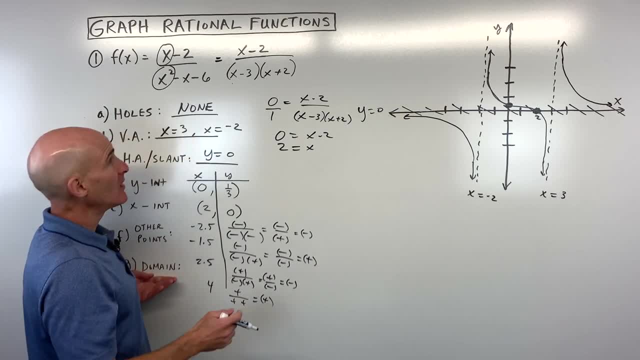 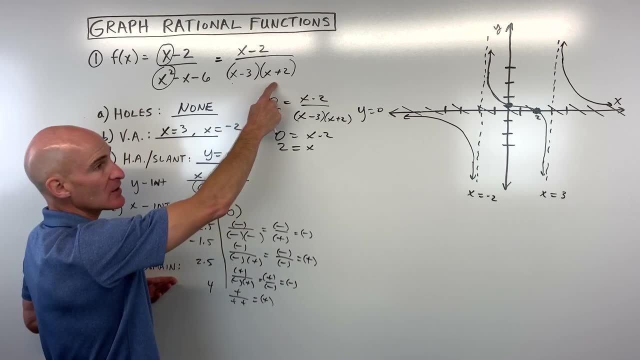 The only other question your teacher might ask is like: what's the domain? What's the positive to negative? Well, that's different now of this rational function. And again we said that the denominator can't be zero. Okay, So it can't be three or negative two. 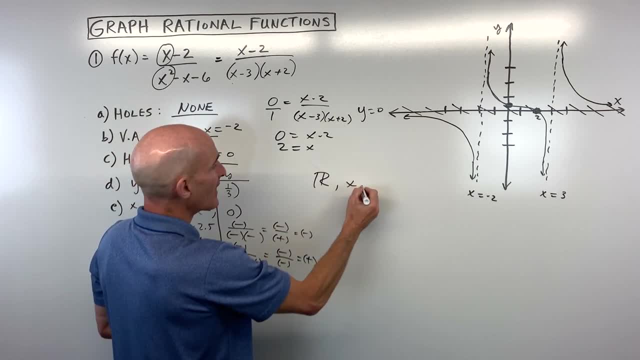 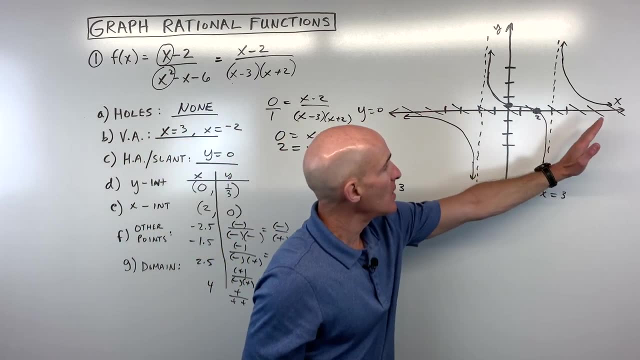 So you could say all real numbers- x cannot be, will be say negative two or three. That's one way to do it. Or if you're doing interval notation, you could say it goes from negative infinity up to negative two, not including negative two. 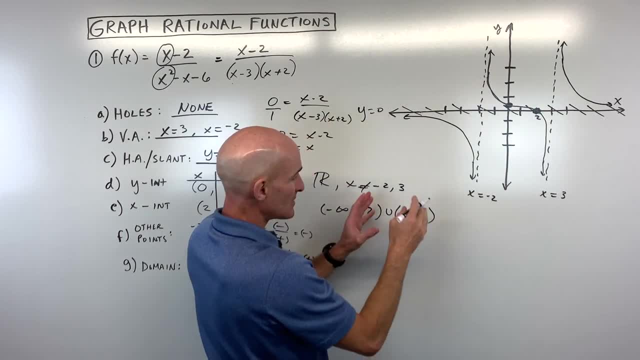 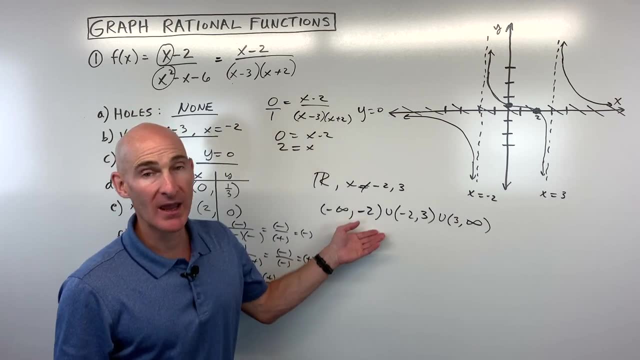 Then it goes from negative two to positive three- not including, That's why we're using the parentheses- And then from positive three on to positive infinity, And that would be your domain. So let's take a look at another example, You know. for example number two, 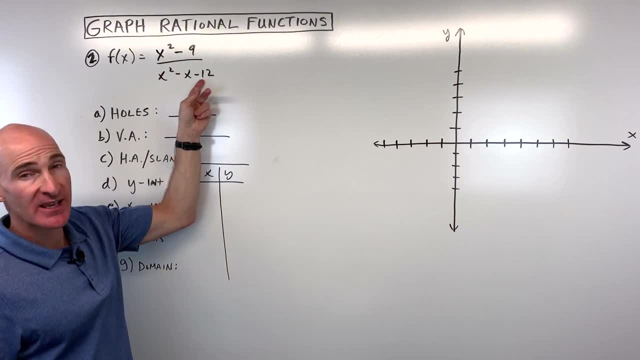 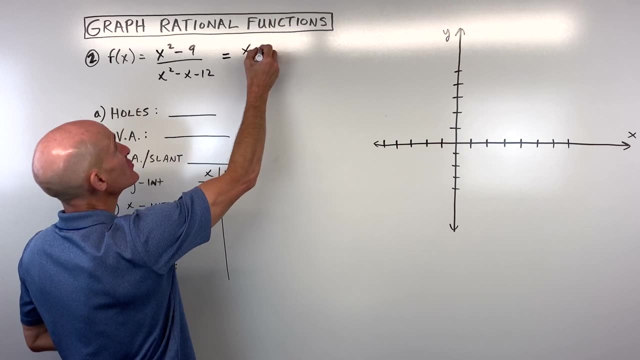 we've got x squared minus nine over x squared minus x minus 12.. So what's the first thing we want to do? We want to factor it as much as we can. So the numerator is the difference of two squares. So we factor that as x minus three, x plus three. 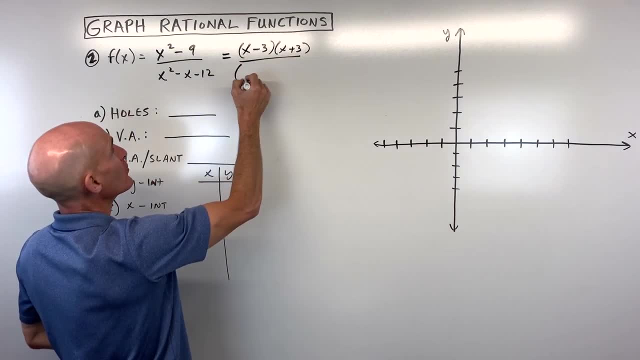 a sum and difference pattern. The denominator: it's a trinomial, It's a leading coefficient of one. So we say what two numbers multiply to negative 12, but add to negative one. That's going to be. let's see. 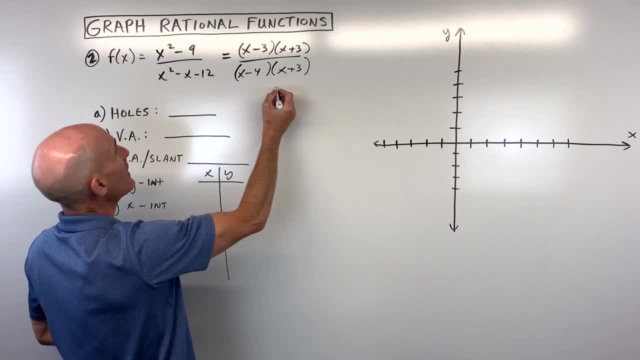 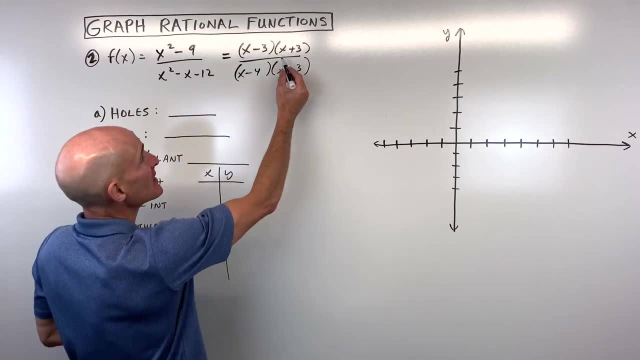 minus four and plus three. And the reason we do that is because we're looking to see if there's any factors in the numerator that cancel the factors in the denominator. And in this case you can see the x plus threes are going to cancel. 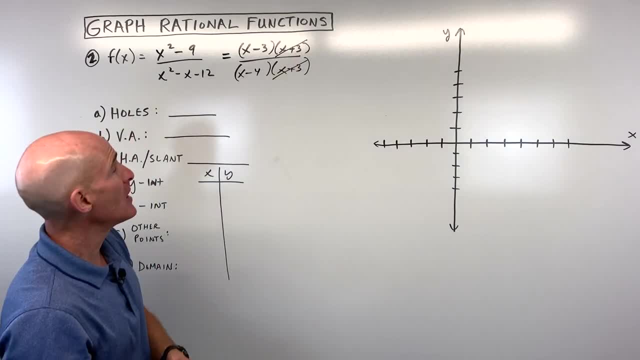 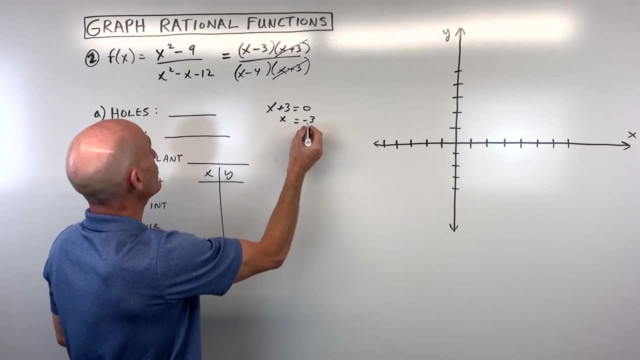 And what that tells us is that we're going to have a hole in our graph. If you set x plus three, equal to zero, and solve, we get the x coordinate of the hole, which is negative three To find the y coordinate of the hole. 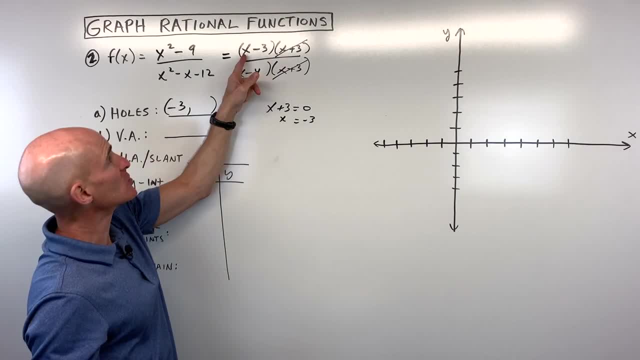 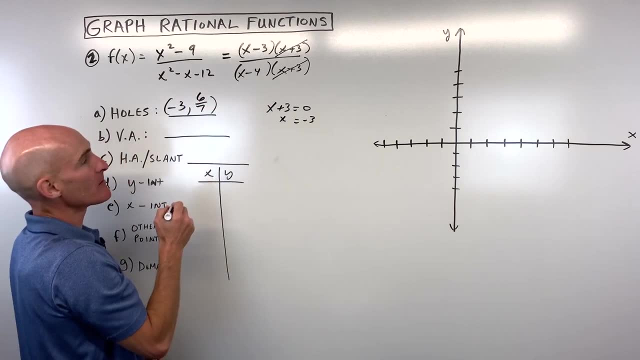 we take the negative three and we put it back in to what's left here. So we get a negative six over a negative seven, which is six sevenths. So let's go ahead and plot that on our graph. So negative three, six sevenths is almost up to one. 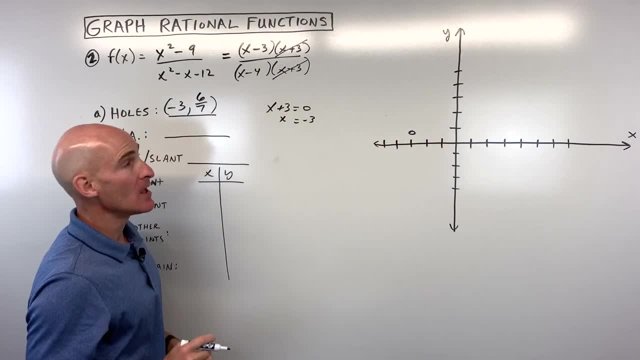 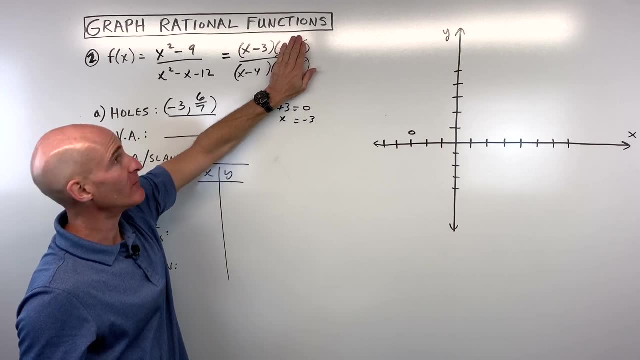 but not quite. So we'll just write about here. That's our hole. Now. as far as the graph is concerned, it's basically like graphing: y equals x minus three over x minus four, because these factors cancel. The only added feature is that there's going to be 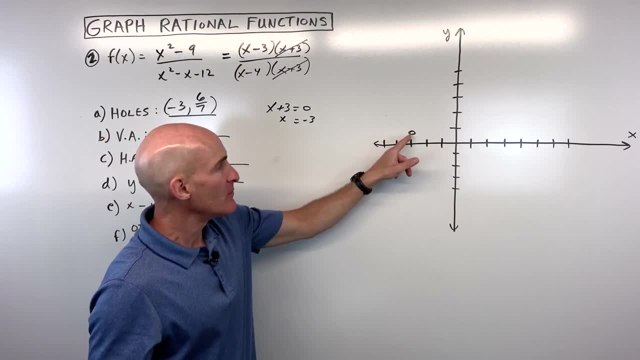 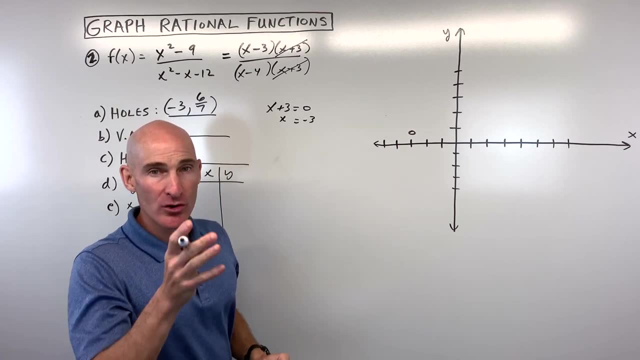 a hole in the graph. Now, if you graph this on your graphing calculator- because this is just like a infinitesimally small, it's just like a little pixel- you're not going to see the hole. But if you go to your table, 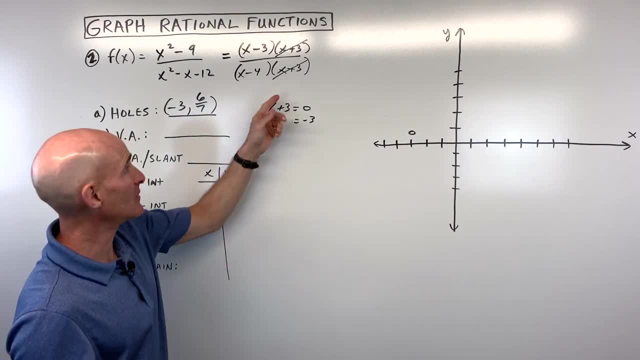 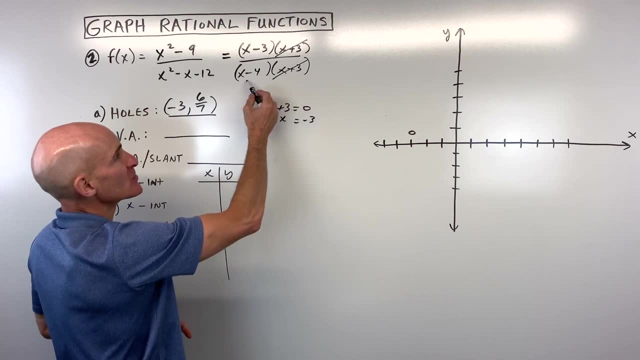 you'll see that there's an error at negative three, Like you. just, it can't be negative three because we can't divide by zero. Now, even before you cancel these factors out like this, you might want to analyze the domain. We said you can't divide by zero. 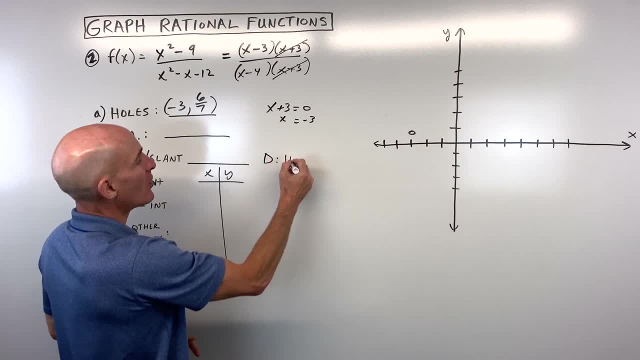 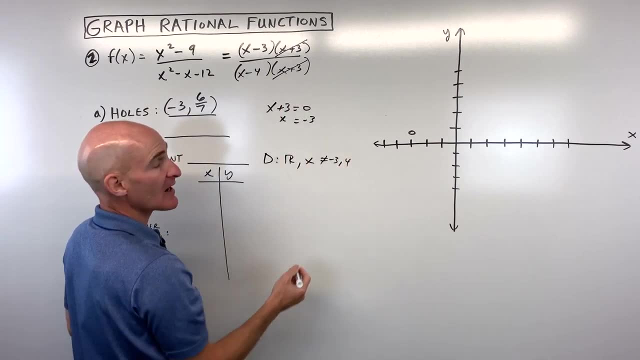 That's undefined. So you can see that the domain, it's going to be all real numbers, but x cannot be negative three and it cannot be four, because that would make the denominator zero right. So you could also write it like this: from low to high: 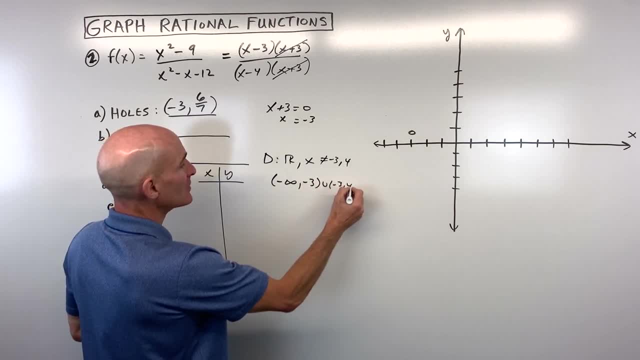 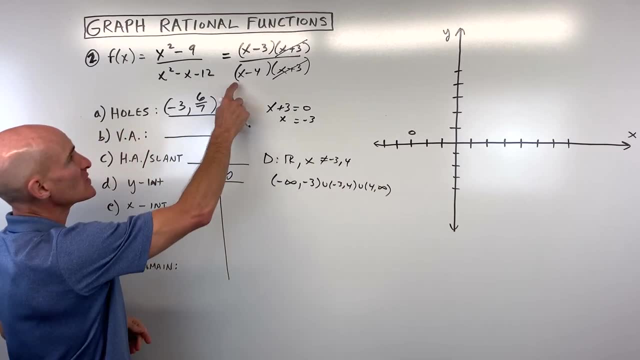 negative infinity to negative three, and then from negative three to four, and then from four on to positive infinity. Okay, now if we talk about the vertical asymptotes, we said we can't divide by zero, right? So what would make this denominator zero? 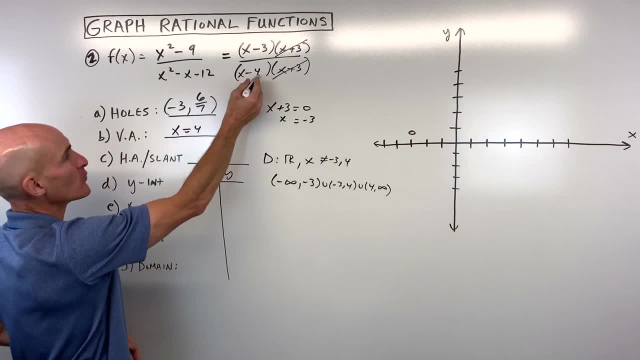 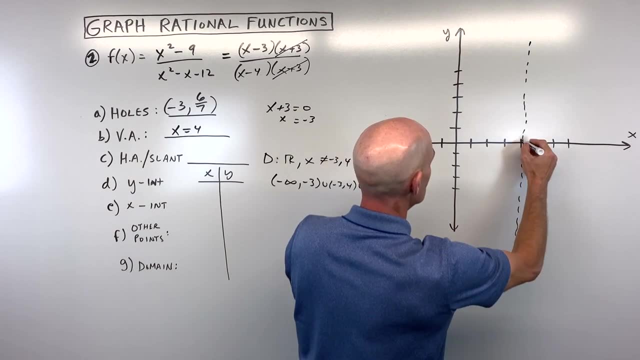 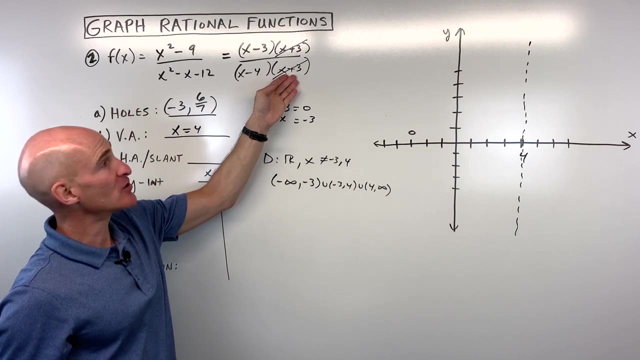 It would be: x equals four, because four minus four is zero. And so we're going to have a vertical asymptote right here at four, Right here at four. So now you might be saying, well, what about here at negative three? That would make the denominator zero. 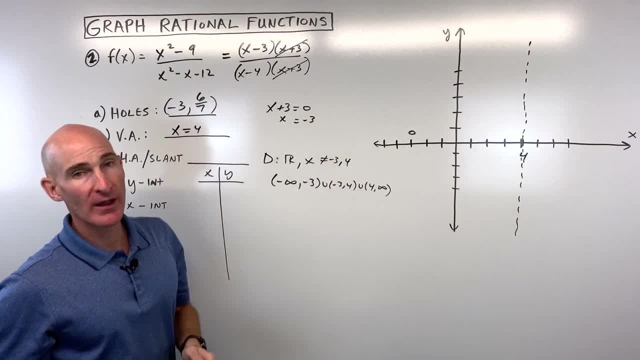 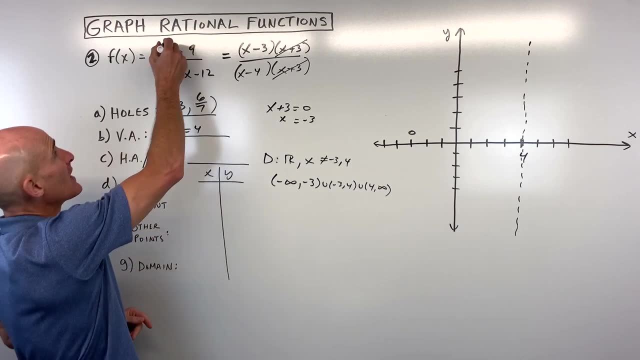 but that's where our hole is located. So it's either going to be a hole or a vertical asymptote, but not both. So now let's look at the horizontal asymptote or the slant asymptote. Here's where we focus in on the highest power term. 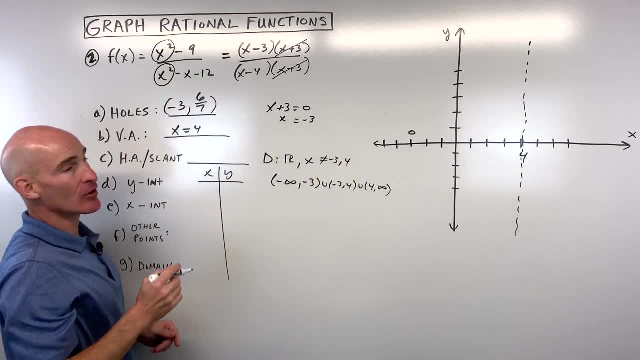 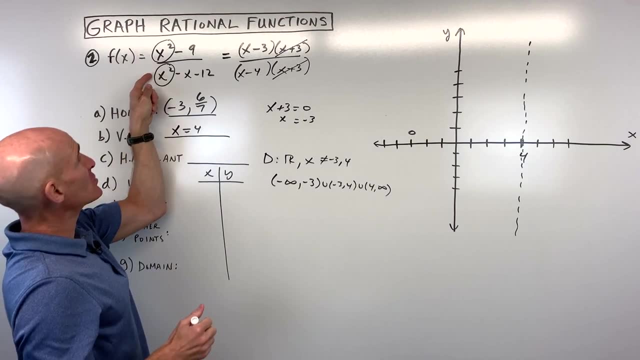 in the numerator the highest power term in the denominator. Now if it's a tie like see how these are both x squared, then what we do is we take the ratio of the coefficients in front of those variables. So in this case this is understood to be a one and a one. 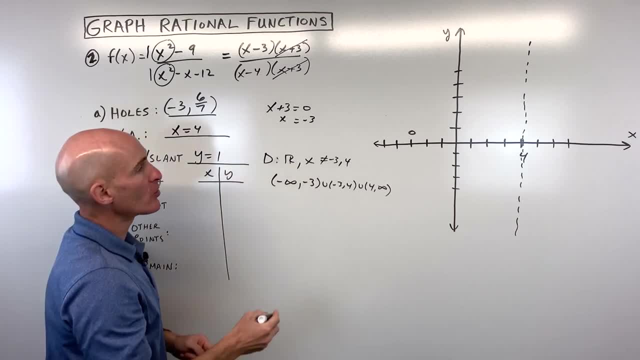 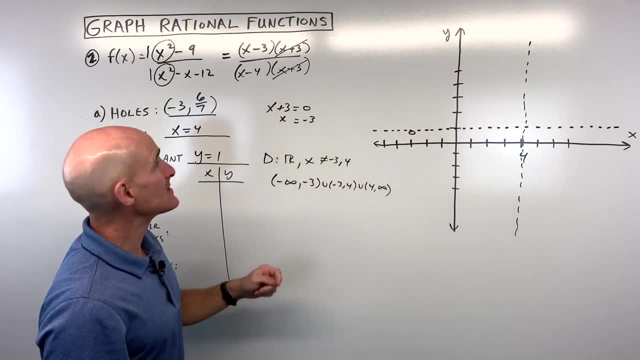 So one divided by one is one, And our horizontal asymptote is going to be right here at: y equals one. Now you might be saying: Mario, why is that? Well, what happens? Well, what happens, What happens is x gets bigger and bigger. 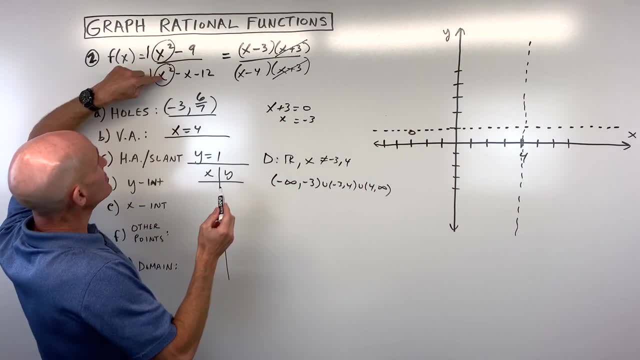 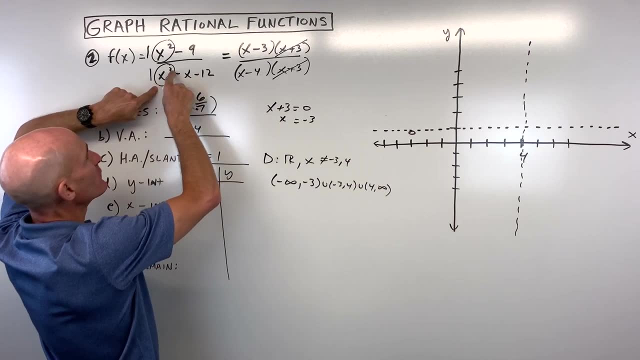 Like, say, if we put x as 100 in way over here to the right, This term is going to go faster than this term. This term is just going to stay at negative 12.. So as this gets bigger and bigger, this term is going to be much more influential. 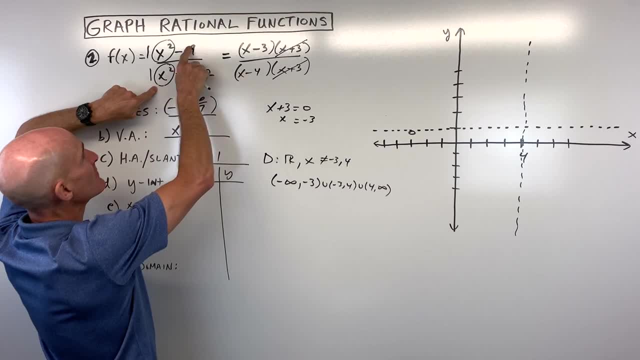 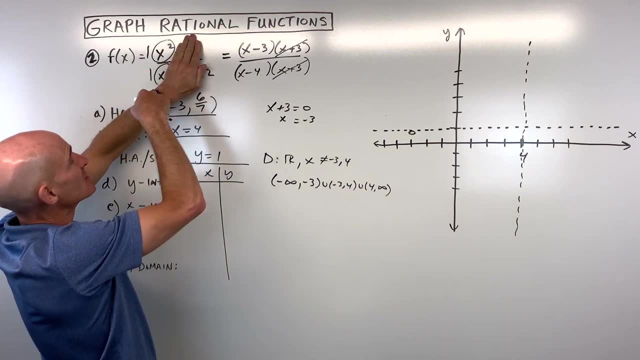 These are going to not really have much of an effect as x gets really big. Same thing with the negative nine. So this really reduces or acts like x squared over x squared Anything divided by itself. that's going to cancel out and you're left with one over one. 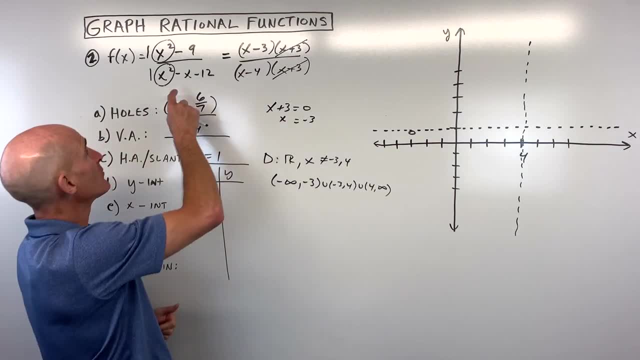 which is the ratio of the coefficients. The last example: remember how the denominator's degree. the denominator's degree was higher. That's y equals zero. You're going to get, it's going to get closer to zero, which is the x-axis. 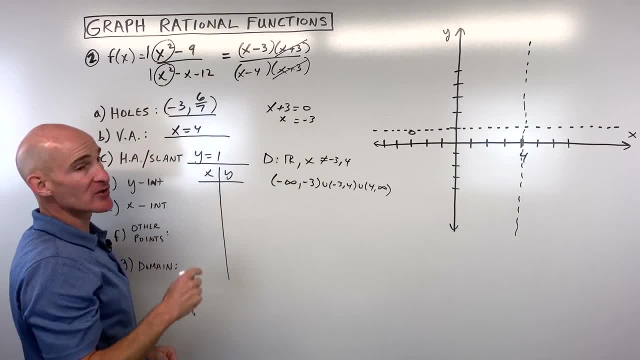 And we're going to do some examples where the numerator's power is greater by a power of one, And that's where we're going to get the slant asymptote. So that's coming in the next examples. So now for the y-intercept. what we do is we set x equal to zero. 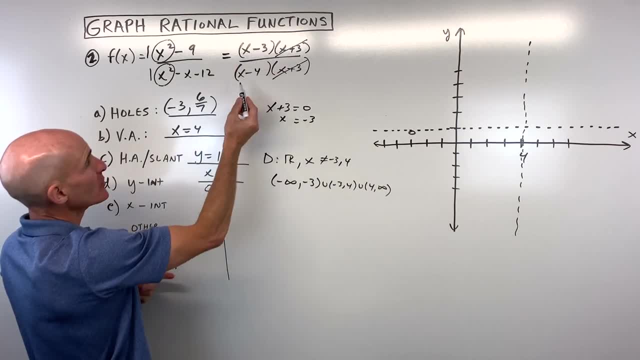 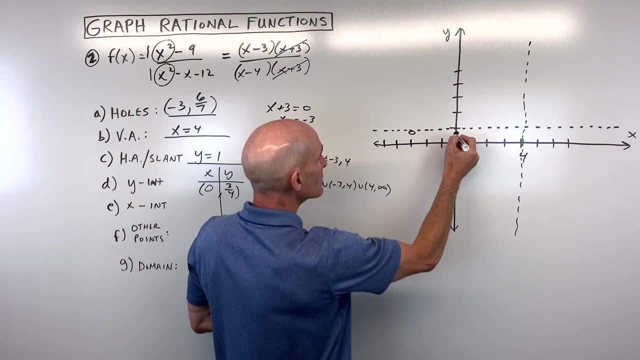 So if I put zero in for x, that's going to be negative three over negative four, which is three fourths. So that's going to be right about here. Now you might be saying: you know why didn't I use this one? 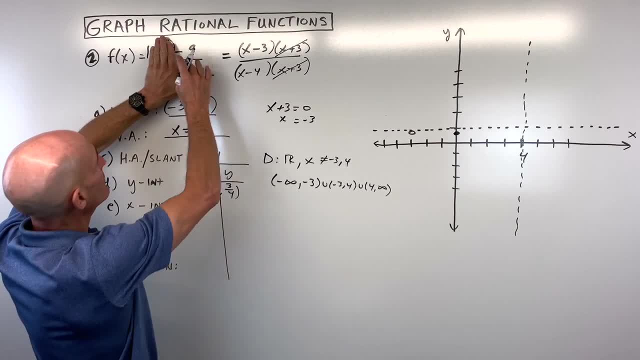 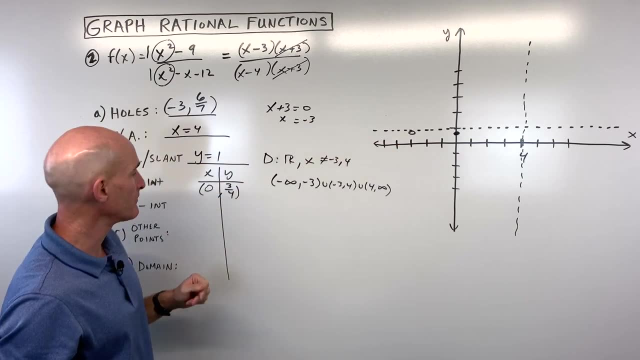 I could use this one too. If I put zero in for x, all these are going to cancel out Negative nine over negative 12 is also three, fourths, Just that. the graph's basically going to look like this, with the added feature of having that hole there. 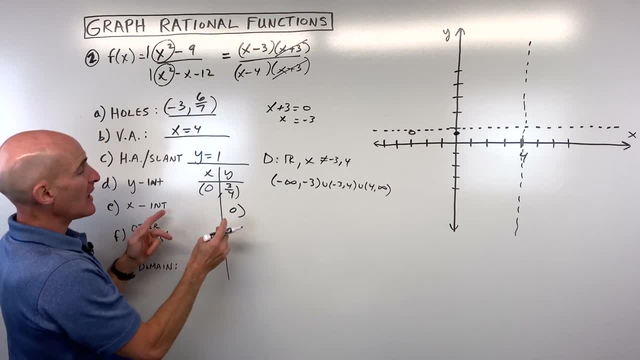 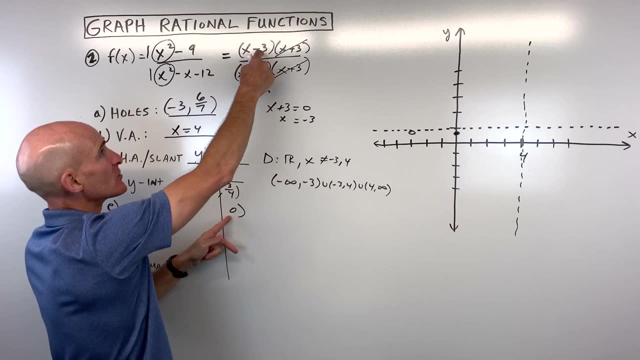 Now, with the x-intercept, we set the y-coordinate to zero. And again, remember the shortcut- is the only way that y is going to be equal to zero is if the numerator's factors are equal to zero. So if I set x minus three equal to zero, 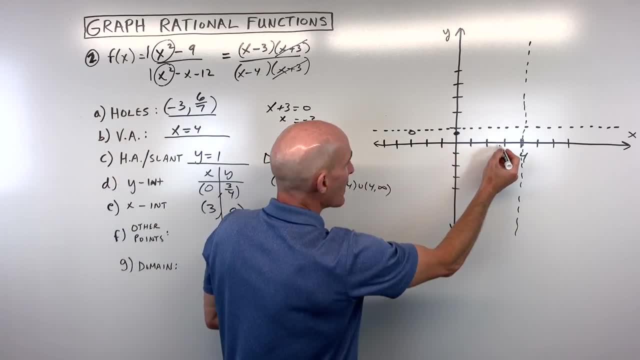 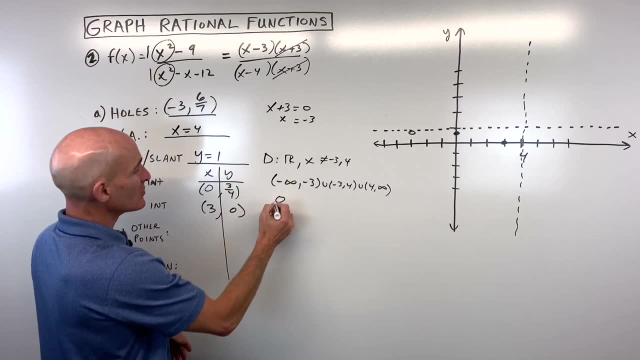 I'm going to get x equals three, which, on my graph, is going to be right here. Now you might be saying: oh, I don't like that method, Mario. So you could say: well, okay, y is equal to zero. 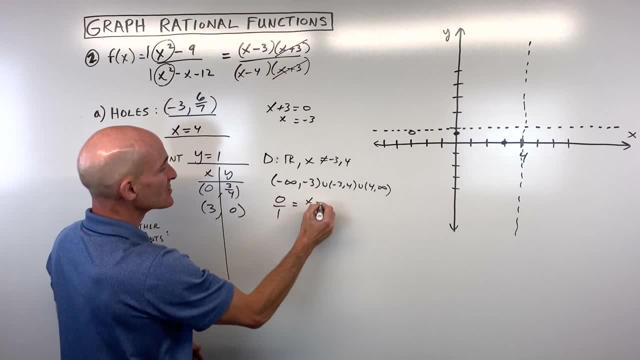 which is like zero over one. Remember. our graph is going to look like this: reduced function: x minus three over x minus four. You can cross, multiply, remember, on the diagonals: zero times anything is zero. x minus three times one is itself. 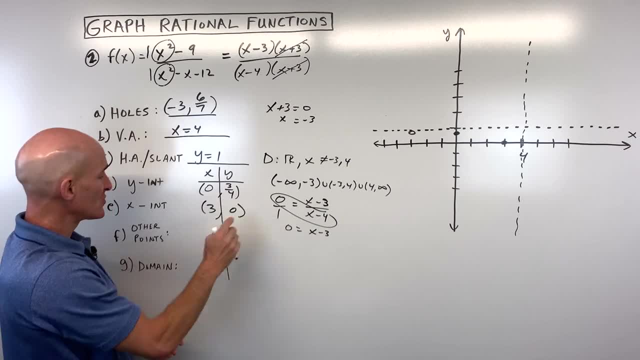 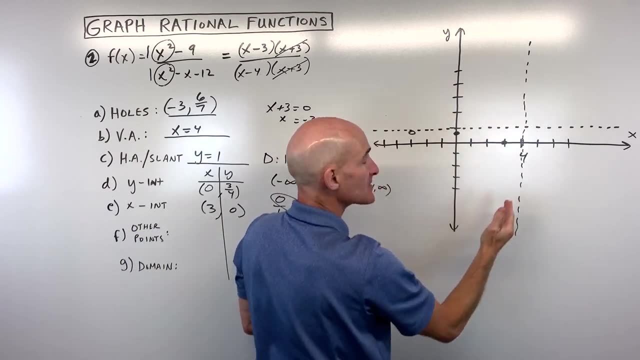 And if you add three, you can see you're getting x equals three. Some students like this much better. Now we need to plot some additional points, but remember we can't go through this vertical asymptote. It's like a brick wall. 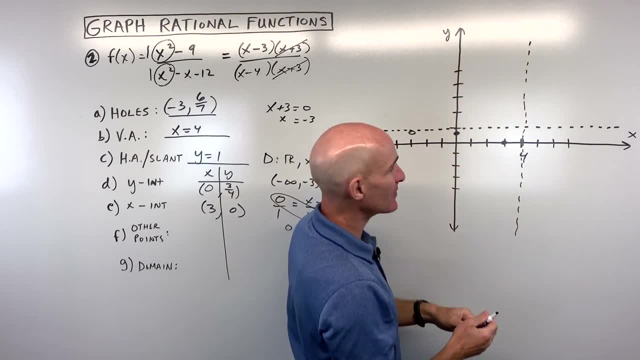 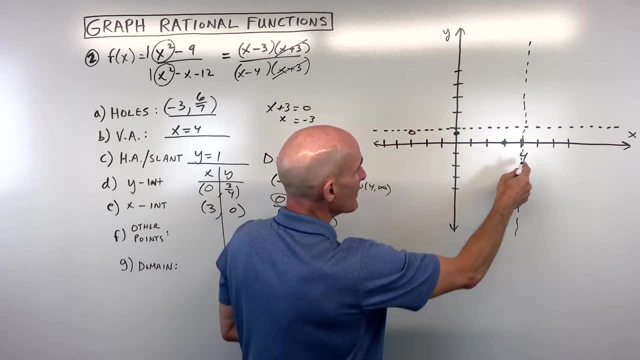 Either graph either has to go up towards positive infinity, down towards negative infinity, right? How do we know what's happening? Let's pick some points on either side. Let's pick 3.5 and like 4.5, or maybe even five. 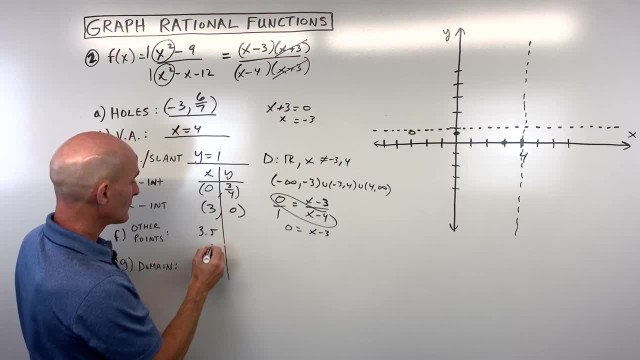 So let's do 3.5 first. So I plug in 3.5, I'm going to get a positive in the numerator. This is the sign analysis: 3.5 minus four. I get a negative in the denominator. 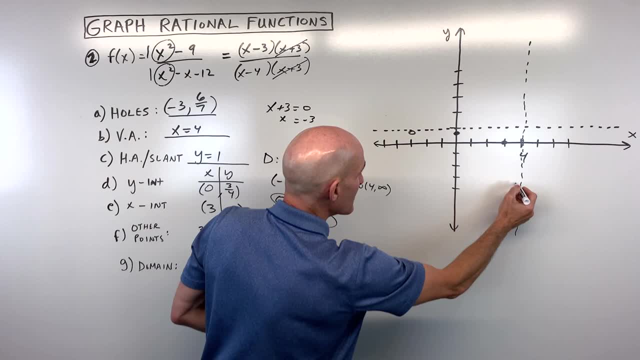 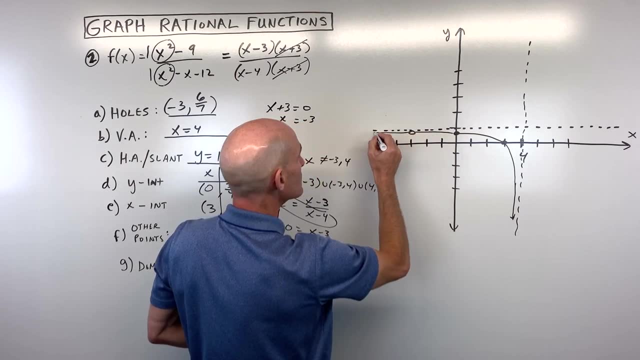 A positive divided by a negative is a negative, which kind of makes sense. This is going down, down, down, So you can kind of see this graph is going to look like this: OK, and you've got that branch. Now if we do five, that's going to give us a positive two. 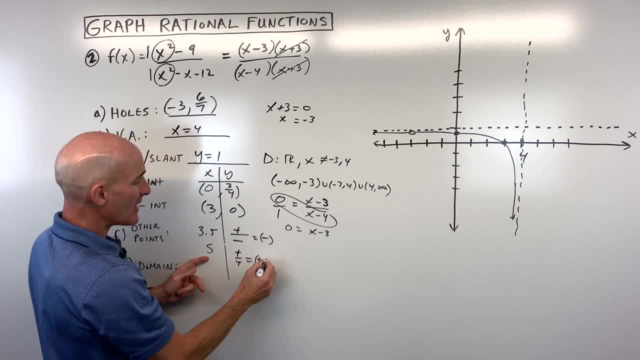 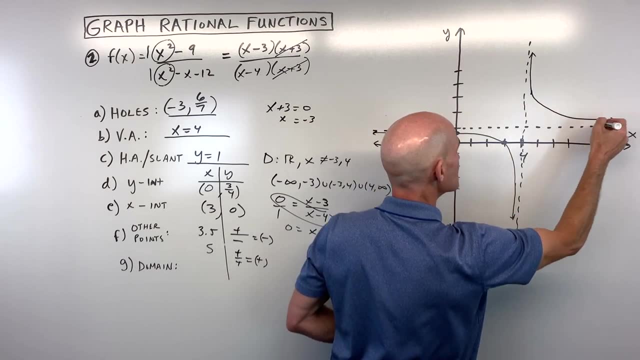 over a positive one. Positive divided by a positive is a positive which tells us from this direction we're going to be going up towards positive infinity. and then we're going to approach that horizontal asymptote as we go to the right and you've got a good sketch. 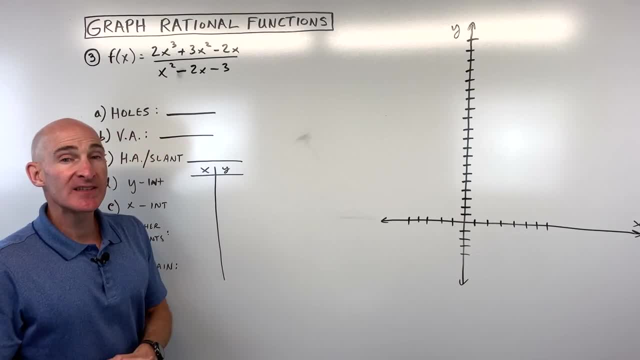 Let's take a look at another example. OK, let's take a look at example number three. now We've got this polynomial divided by a polynomial, a rational function. First thing we want to do is factor right. So in the numerator it looks like we can factor out an x. 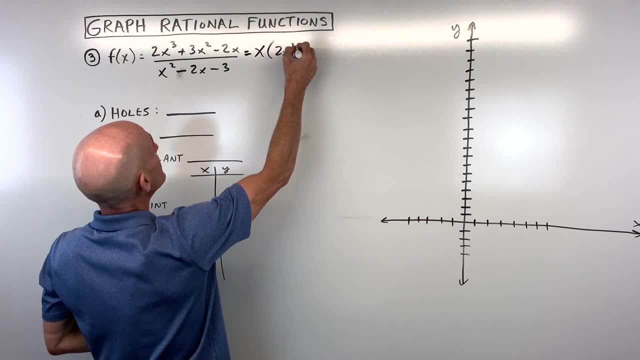 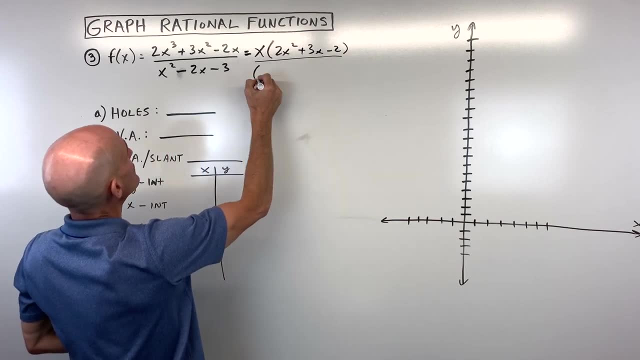 as a greatest common factor, and if we do that, we're going to be left with- let's see two x squared plus three, x minus two, The denominator we can factor. It's going to factor to x minus three and x plus two. 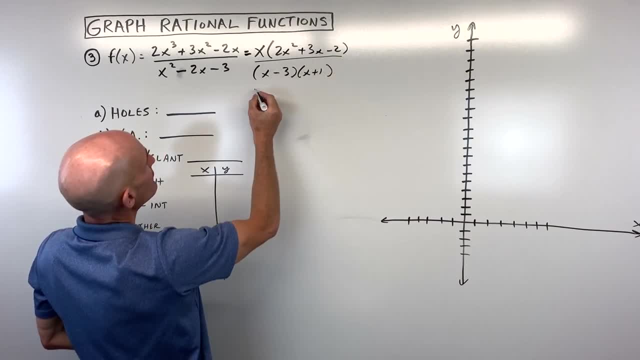 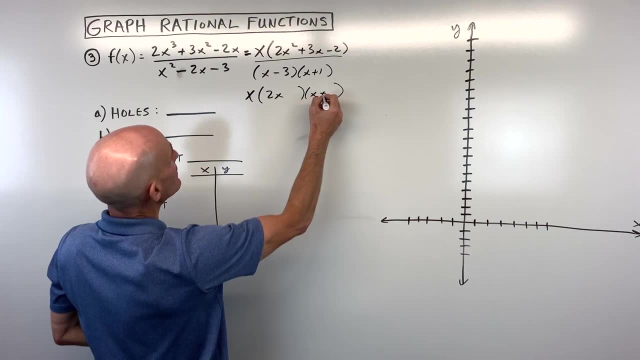 Plus one. This trinomial we can factor a little bit further. So that's going to factor as let's see two x and one x, And let's see this is going to be plus two and minus one, And then we have our denominator x minus three x. 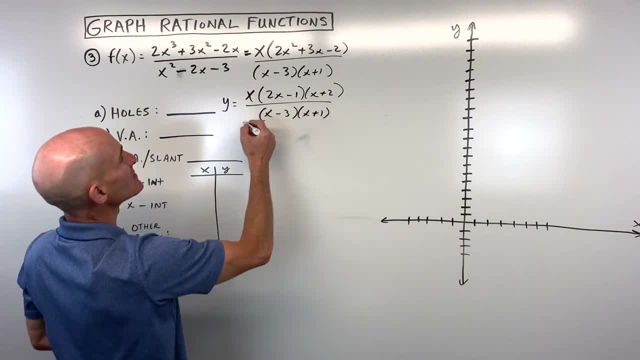 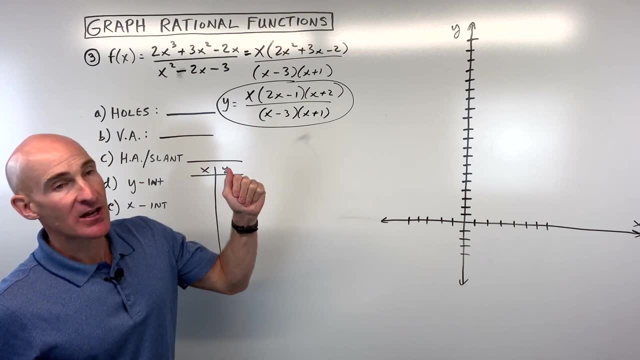 plus one, OK. so basically our equation is going to look like this guy right here. Let's circle that, OK, in factored form. So the first thing we want to analyze is: are there any factors in the numerator that cancel with factors in the denominator? 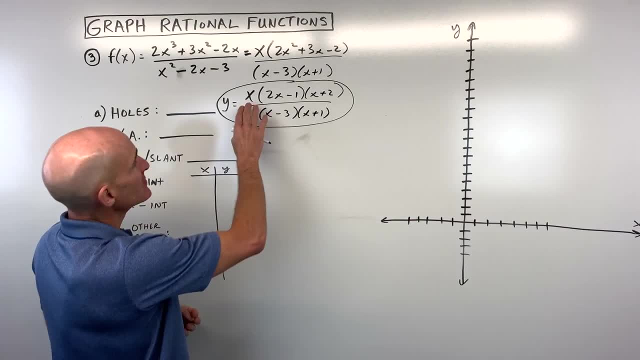 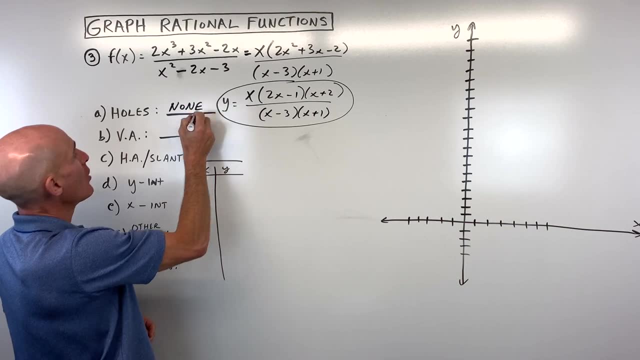 if there are, we know there's going to be some holes in our graph. In this case there's no factors in the numerator that cancel with factors in the denominator, so we're going to say that there's no holes or none. OK, now for the vertical asymptotes. 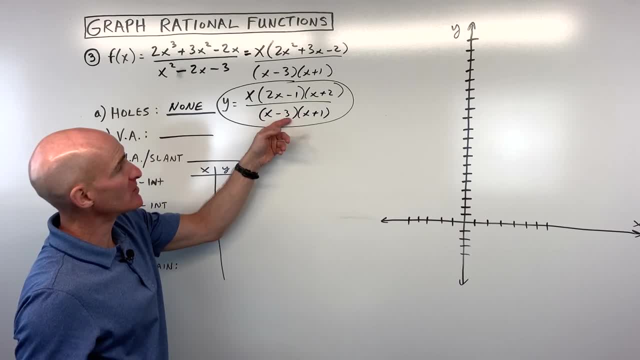 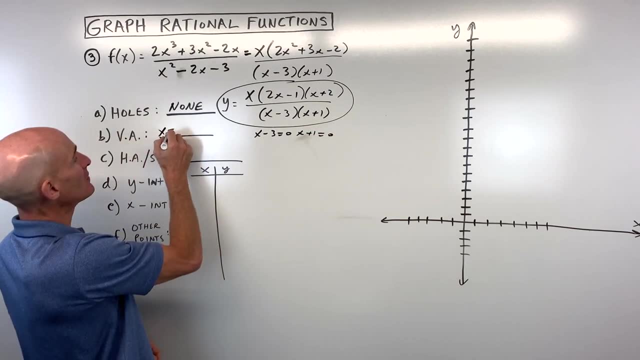 we know we can't divide by zero. So if we set these factors equal to zero in the denominator x minus three equals zero, x plus one equals zero, we're going to get x equals three and x equals negative one. So let's go ahead and plot that on our graph here. 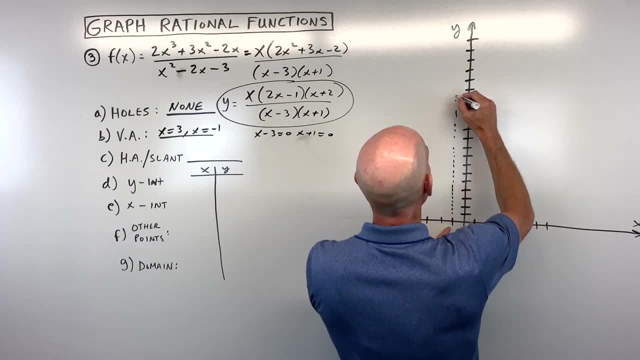 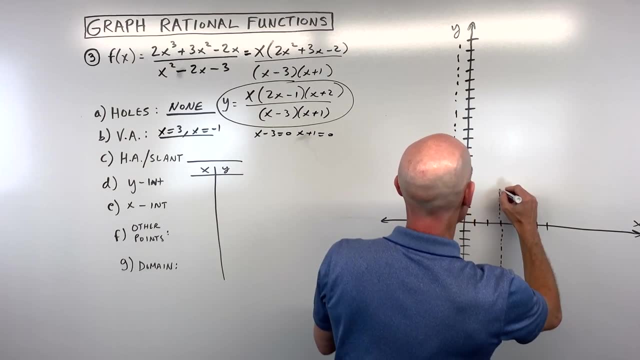 So negative one. Try to be real accurate about this. So here's negative one, and x equals three. It's going to be right here, Just trying to draw it as a dashed or dotted line, You won't actually see that on the graph. 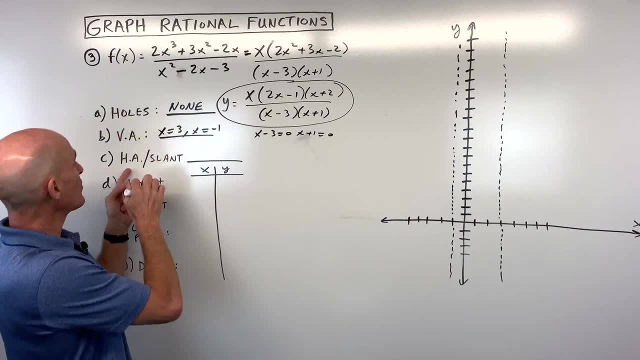 It's just kind of using it as a guide. Now, the next thing we want to do is we want to analyze: do we have a horizontal asymptote or a slant asymptote? Well, in this problem, you see how the highest degree term 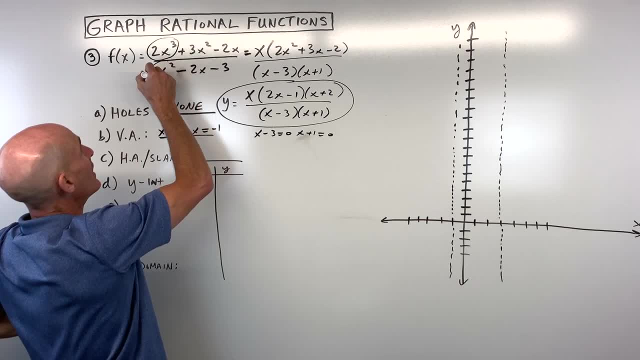 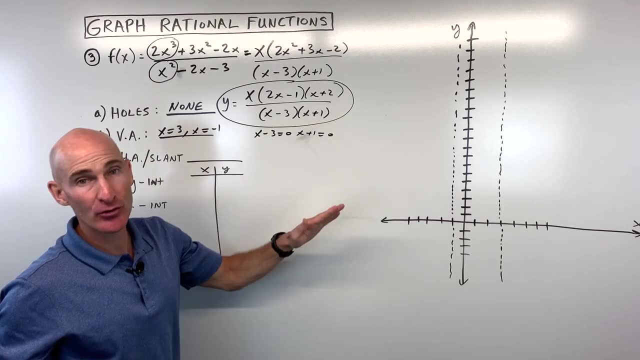 in the numerator is higher than the denominator's highest degree By one. So what that tells us is we're going to have a slant asymptote, like a diagonal, or an oblique asymptote. How do we find the equation of that oblique asymptote? 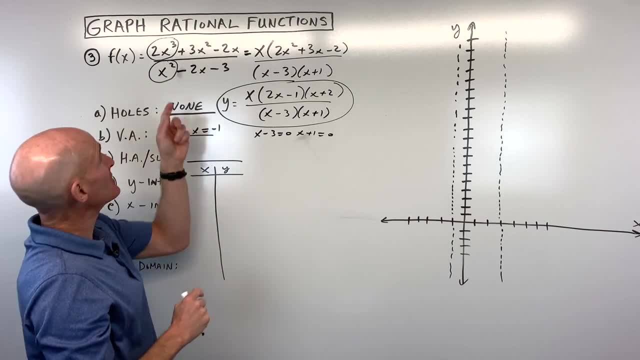 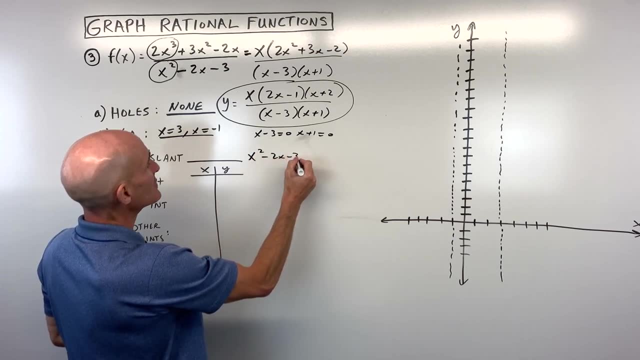 or slant asymptote. We're going to do long division, So I'm going to take the numerator divided by the denominator. So we're saying: how many times does x squared minus 2x minus three go into 2x cubed plus 3x squared minus 2x plus zero? 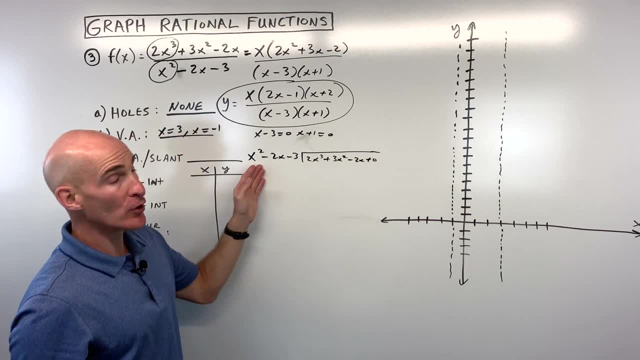 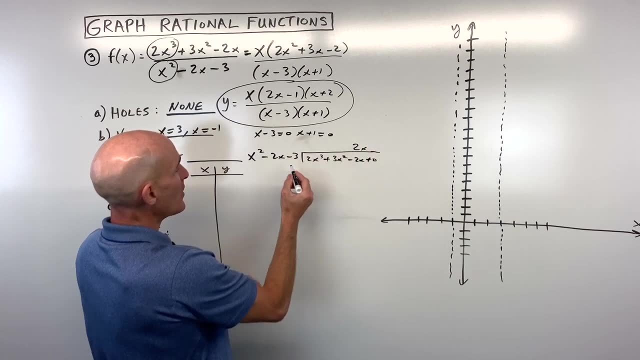 OK, so you probably learned this before. polynomial long division: How many times does x squared go into 2x? cubed, That's going to be 2x times. I'm going to distribute the 2x to all three of these terms. 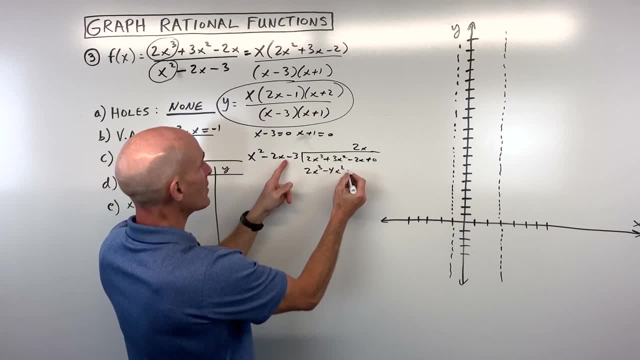 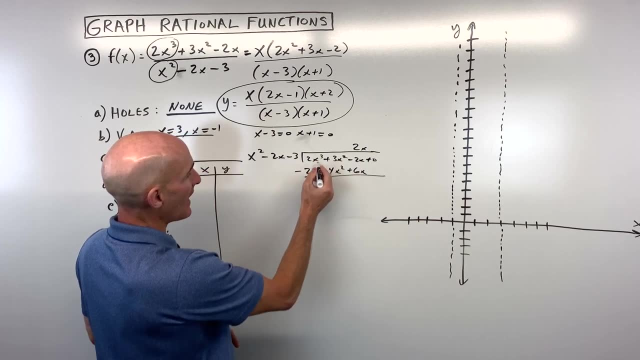 That's going to give us 2x cubed minus 4x squared minus 6x. You can subtract, or what some students like to do is change the sign to the opposite and add. So that's going to give us 7x squared plus 4x plus zero. 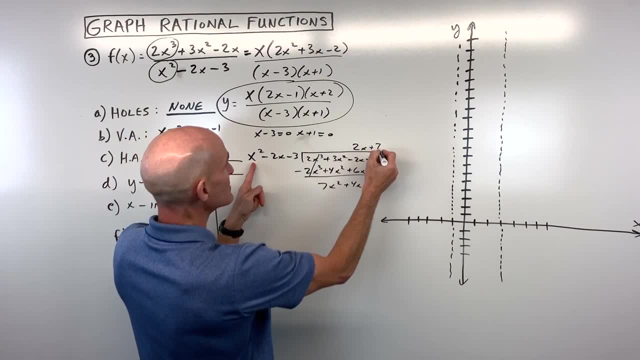 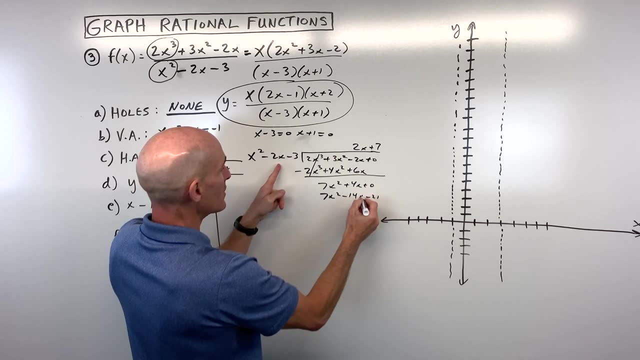 How many times does x squared go into 7x? 7x squared, that's seven times. If I distribute the 7 to all three of these terms, I get 7x squared minus 14x minus 21.. If I subtract or change the signs to the opposite and add: 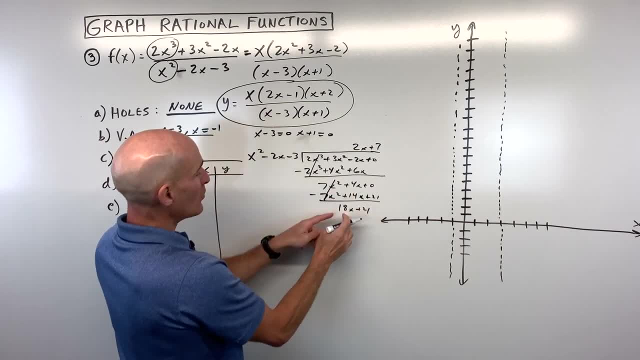 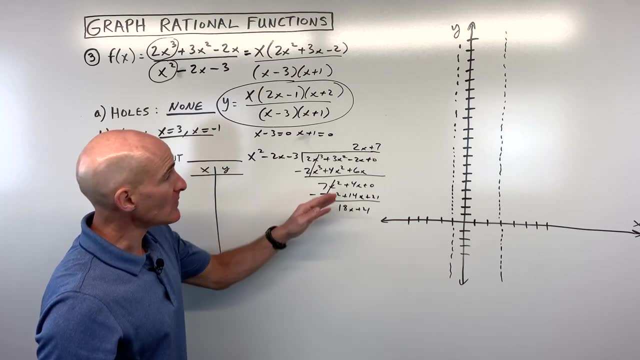 that's giving us 18x plus 21.. And when this degree x to the first is lower than this degree x squared, that's our remainder. We don't have to worry about the remainder. So our equation of our slant asymptote: 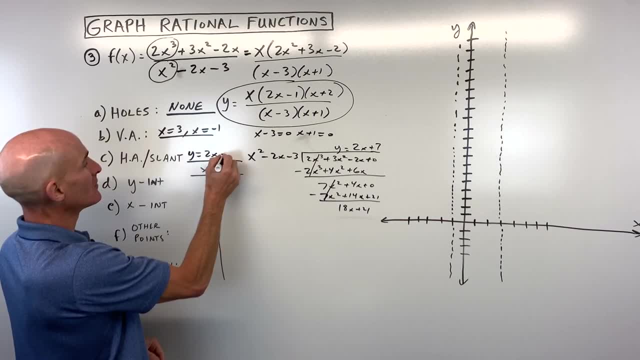 is going to be: y equals 2x plus 7.. So that means it has a y-intercept of 7.. 1,, 2,, 3,, 4,, 5,, 6,, 7, right about here. 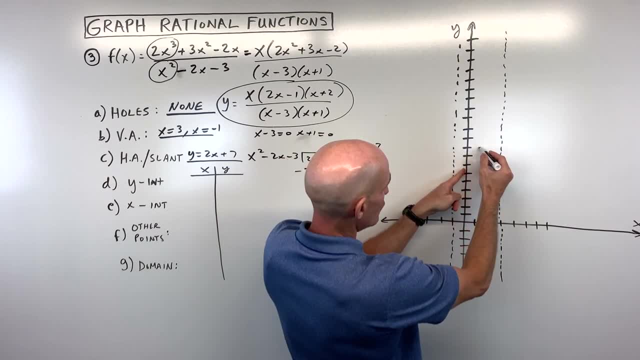 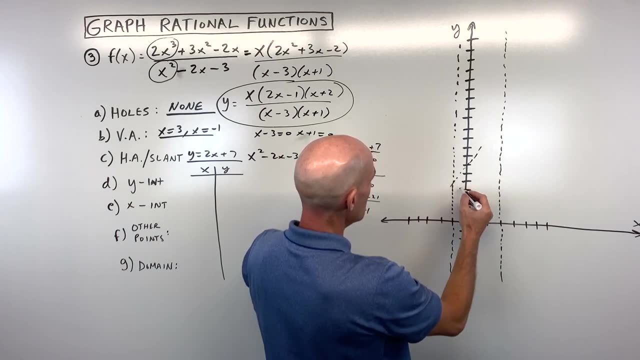 A slope of 2, which means I'm going to go rise 2,, run 1,, like this. So down 2, over 1,, cross right about here. Let's repeat that: down 2, over 1,, right about here. 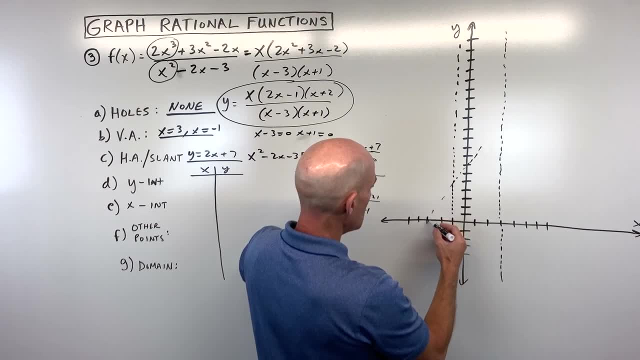 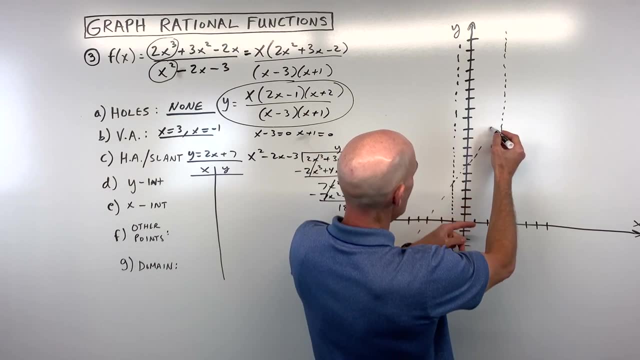 Down 2, over 1,. right about here. Let's see: down 2, over 1, right about here. So, roughly, let's repeat this a little bit here: up 2, over 1, and up 2, over 1,, up 2.. 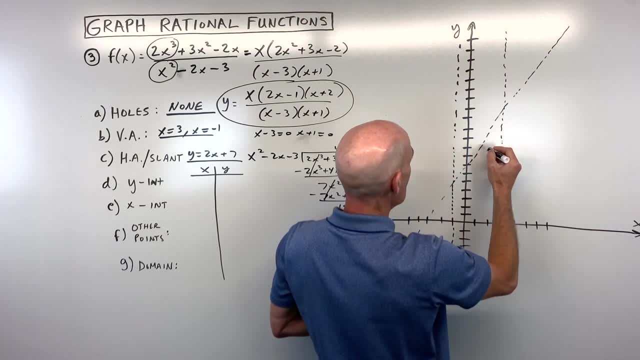 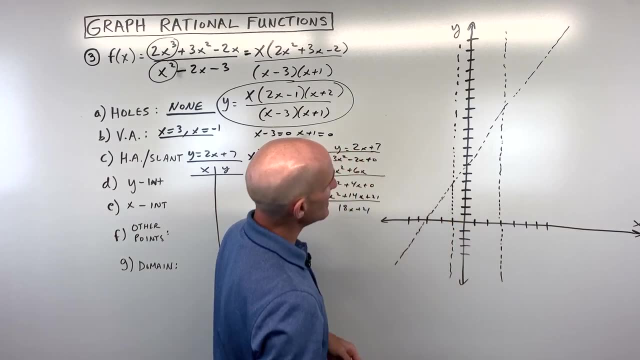 Okay. so basically, like this- I'm trying to be accurate: We don't have graph paper here, I don't have graph paper on this screen, here, on this board, So we can just kind of estimate like that. Okay, so now let's focus on the y-intercept. 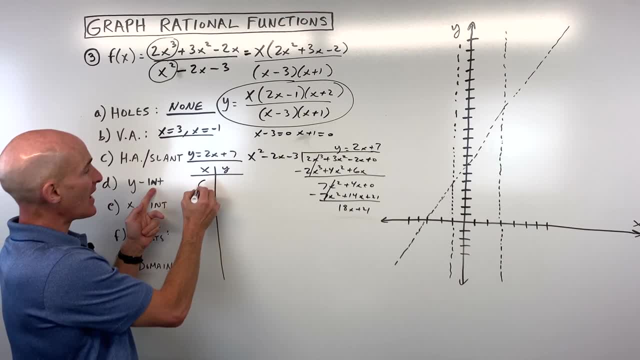 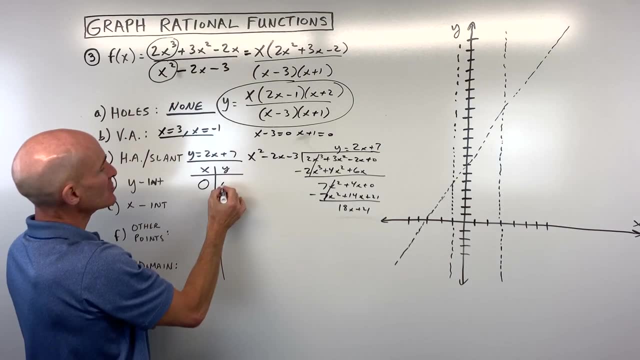 and the x-intercept. So to find the y-intercept, we set x equal to 0. And if we put x equal to 0, you can see that it's going to be 0 over negative 3, which is just 0.. 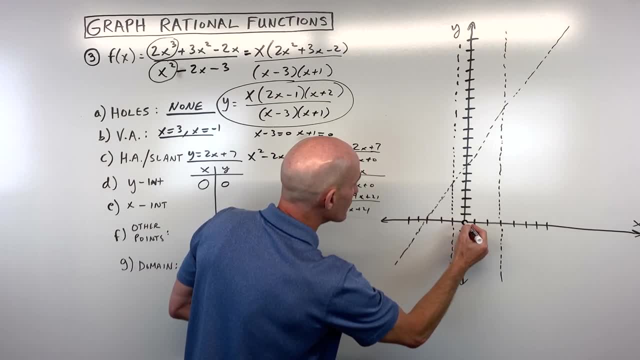 So that tells us it's going to go right through the origin here. Let's put a point right there. And the x-intercept? we're going to set y equal to 0.. Now remember when y is equal to 0,. 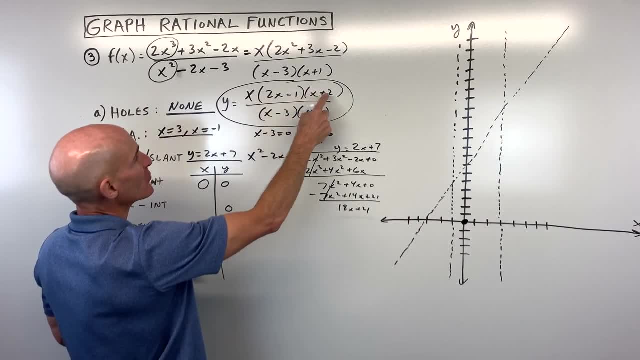 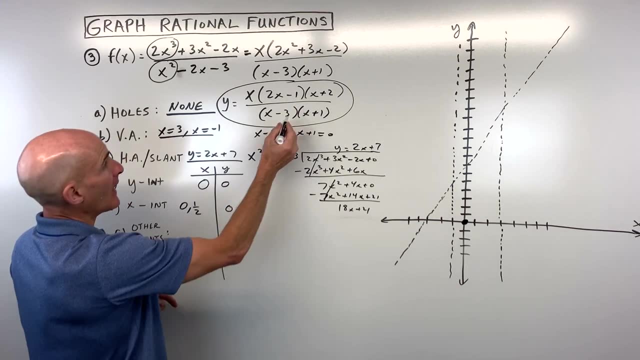 the only way that y is going to be equal to 0 is if the numerator's factors are equal to 0. So that's going to occur at 0, 1 half and negative 2.. So let's see, let's plot that. 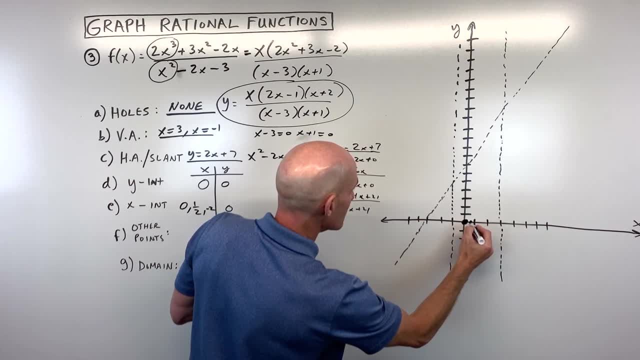 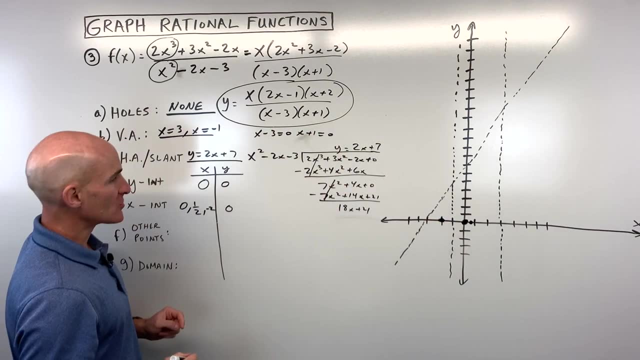 So 0,, 1 half, which is right about here, and negative 2, which is right about here. Okay, so that's interesting, And now some additional points. Now we want to plot some points on either side of the vertical asymptotes. 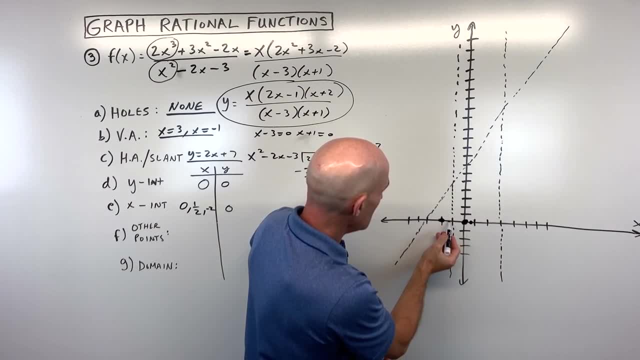 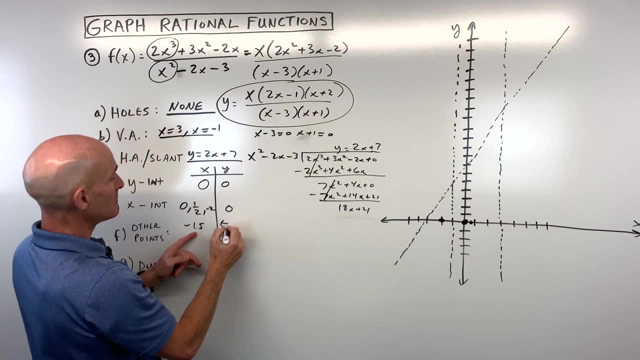 So let's maybe start over here. Let's do a negative 1.5.. So if we plug in negative 1.5, we're going to do our sign analysis. We're going to get a negative. This is going to be a negative. 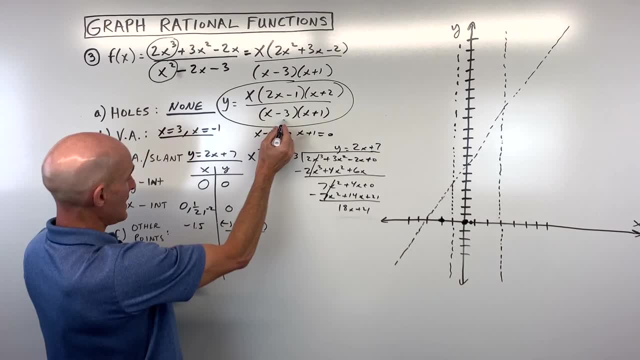 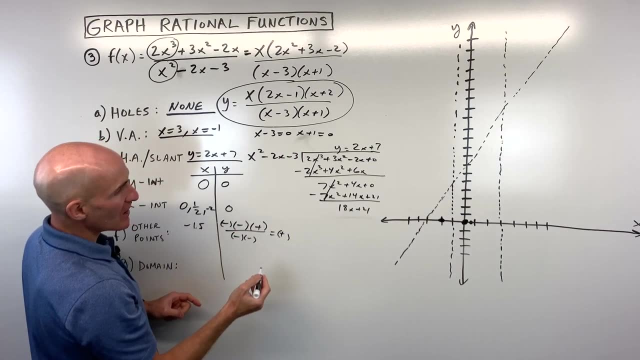 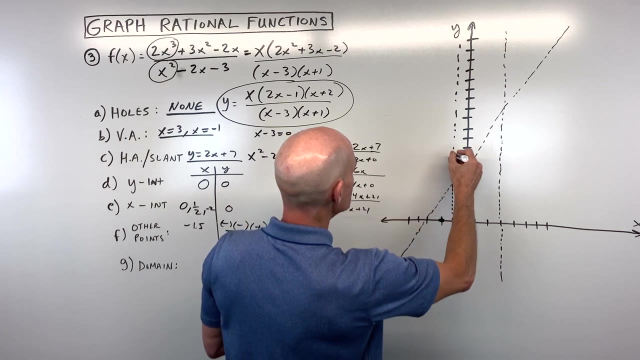 This is going to be a positive, And then we've got a negative and a negative. Okay, so we get a positive divided by a positive, which is a positive. So what that tells us is that this graph is actually going to go up towards positive infinity. 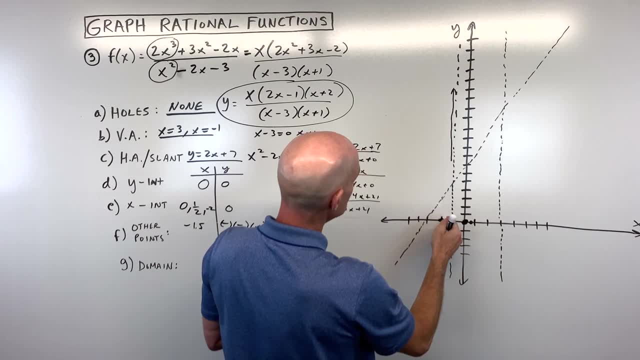 right here, when we're just to the left of this vertical asymptote. So what's happening here? I don't know if you can see. this is this graph is basically going like this: Okay, so as you go here, it's approaching the slant asymptote. 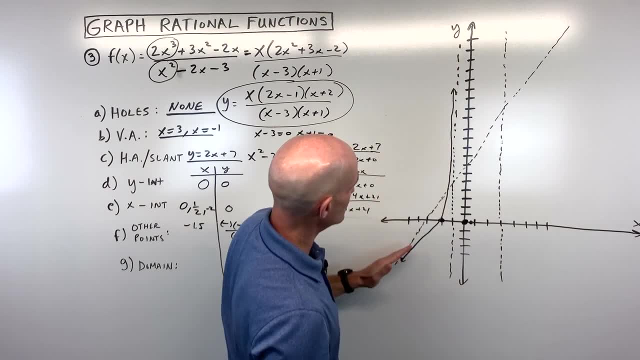 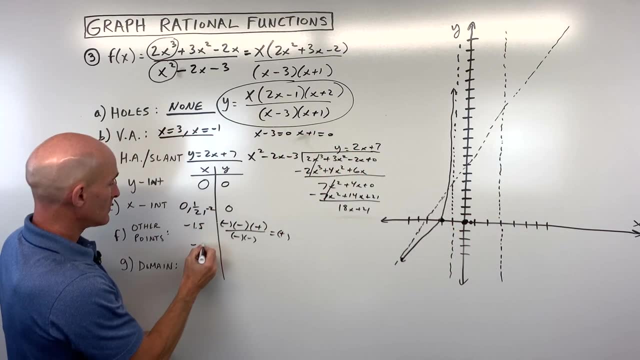 But as it approaches this way, it's going up towards this vertical asymptote. So something like that: Now let's approach this vertical asymptote from this side. Let's say we put in a negative 1.5.. Okay, negative 0.5.. 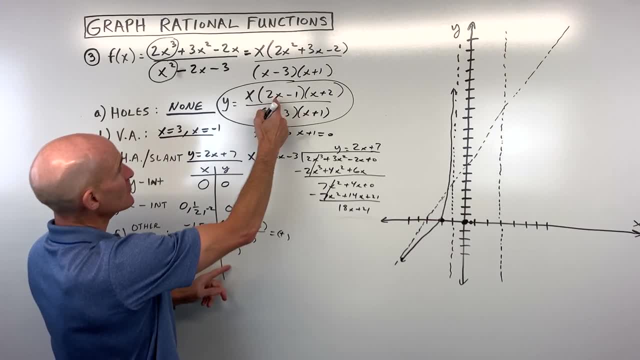 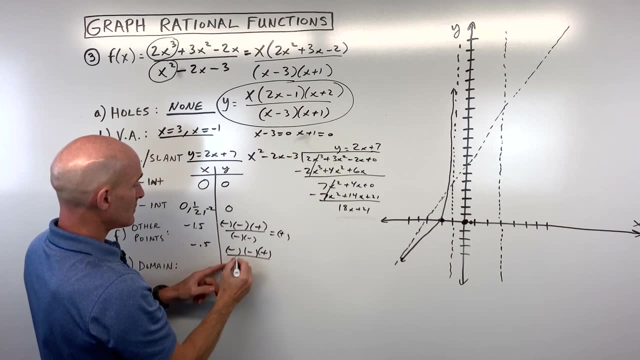 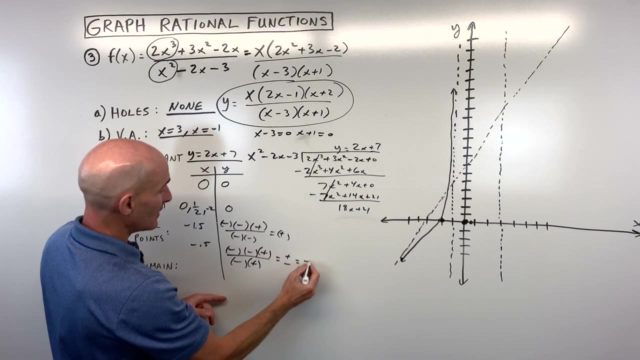 So what happens when we do that? We get a negative. This would be a negative, This would be a positive. again This would be a negative And this would be a positive. So we're getting a positive over a negative, which is a negative. 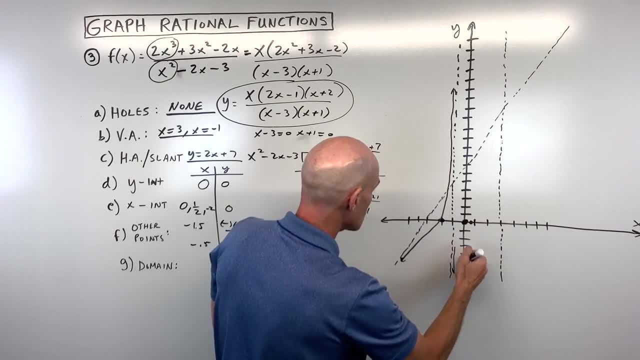 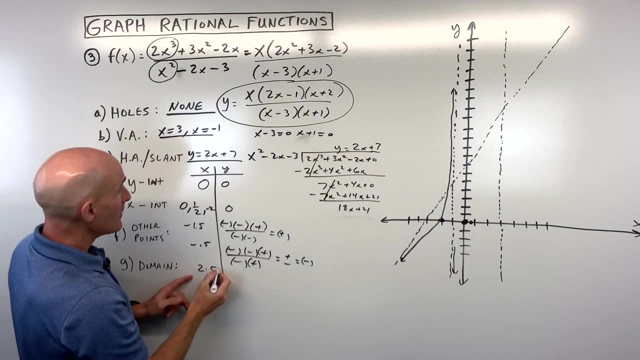 So that means from this side it's going down towards negative infinity. Now, if we approach this vertical asymptote, let's see one, two maybe, like 2.5, what are we getting? We're getting a positive. we're getting a positive. 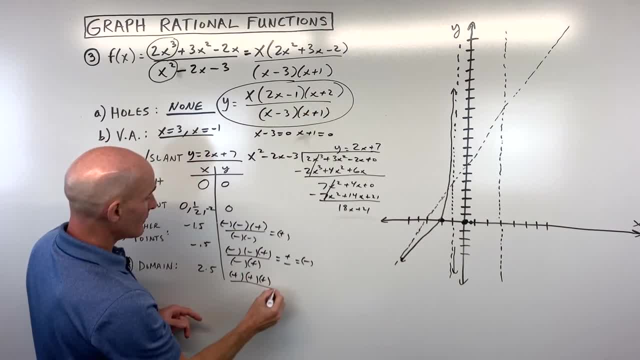 You can get the exact number if you want. This is just a little quicker way of doing it and a little bit more fun too, I think. So this comes out to a negative and this comes out to a positive. So we've got- let's see- a positive divided by a negative, which is a negative. 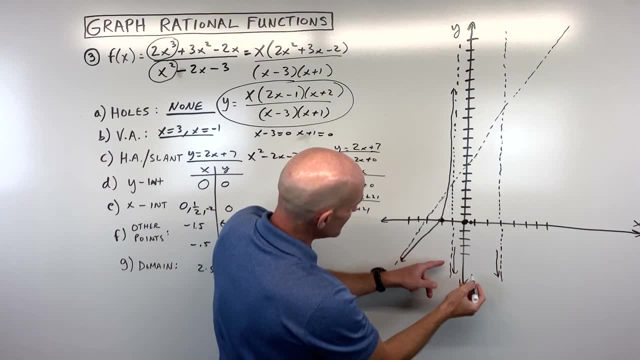 So that tells us on this side we're going down like this. So here you can see that this graph's going something like this: It crosses a little bit the x-axis and it approaches these two asymptotes. Now, if we approach from this side, let's see 1,, 2, 3, let's maybe put 4 in. 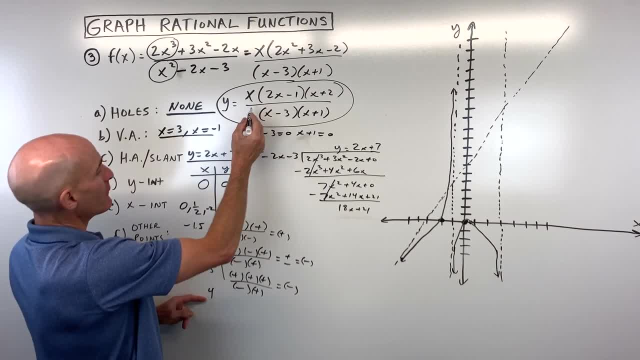 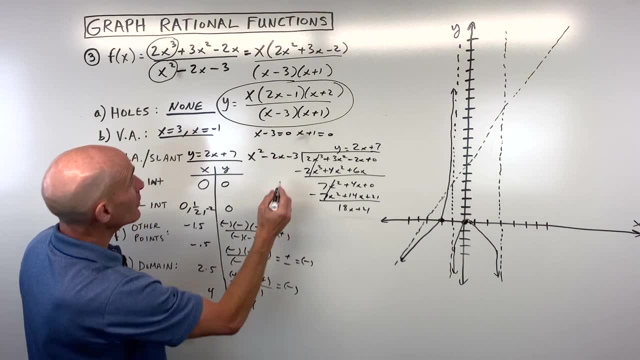 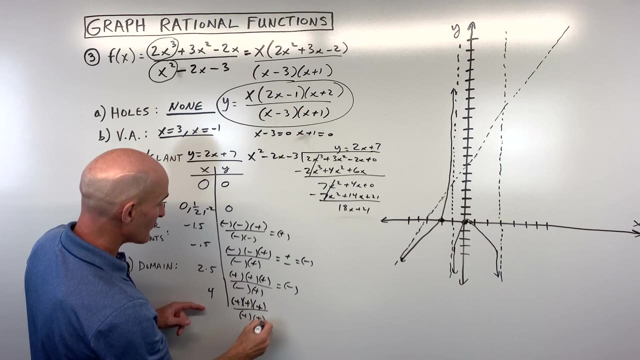 Let's see what happens when we plug 4 in: We get a positive, We get a positive, We get another positive, Okay, and then over here we get a positive and a positive. So you can see, everything is positive. Positive divided by positive is a positive. 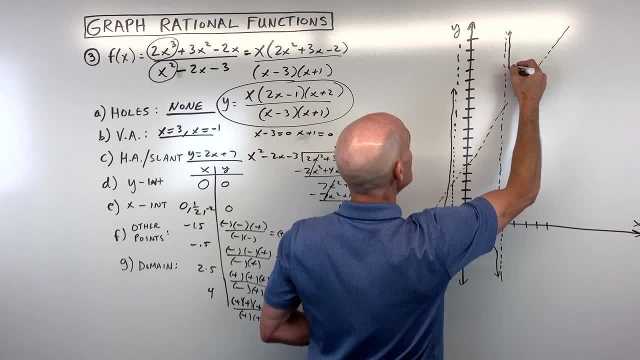 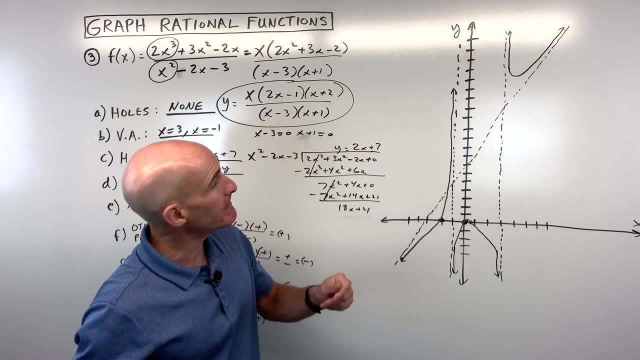 That tells us from this side we're going to be going up towards positive infinity And this branch is going to go approach that slant asymptote. Now here's the questions that people are probably thinking. They're saying: Mario, how did you know? 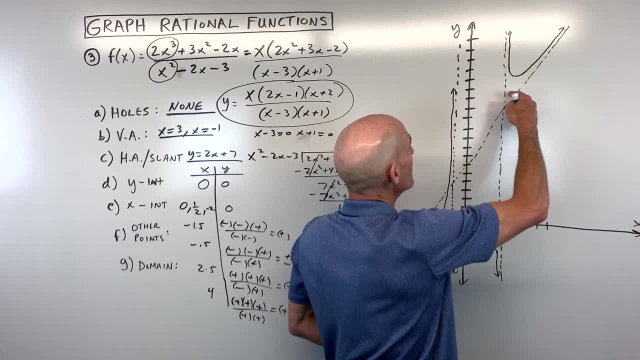 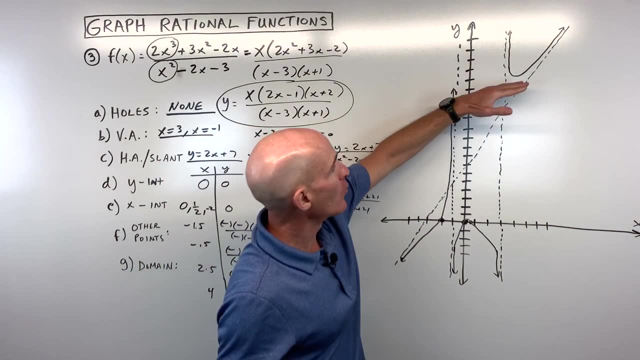 How do you know it bends right here, Like how come it doesn't go all the way down to right here and then go like that? Or how come it doesn't bend over here? This is what you learn when you get to calculus. You're going to learn how to find where the tangent line, the slope of the tangent line, is zero. 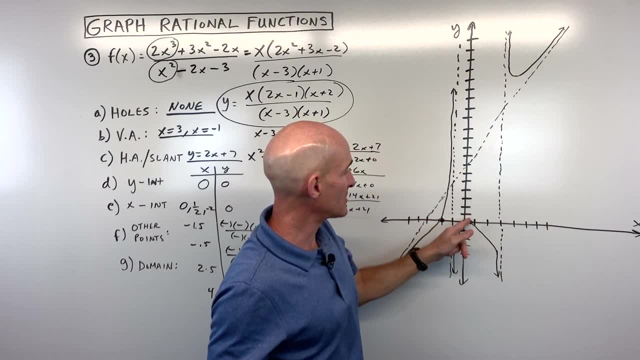 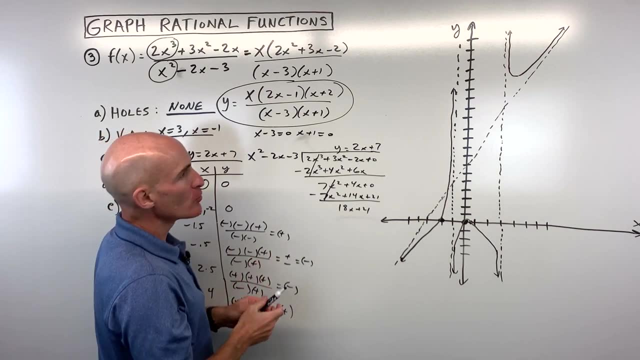 and you're going to be able to find exactly where that minimum is or exactly where this maximum is. But for this video, we're just going to talk about getting a really good sketch, without being super precise, about some of these extramas, as they're called, these bends or maxima. 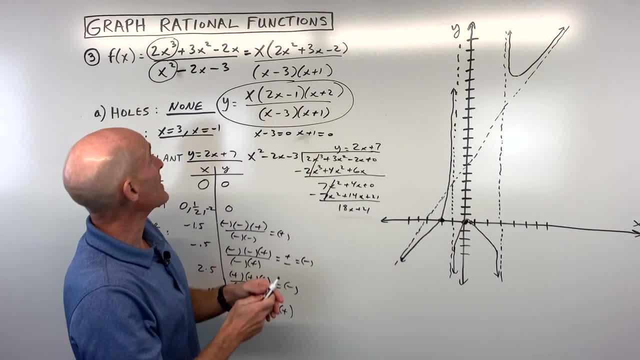 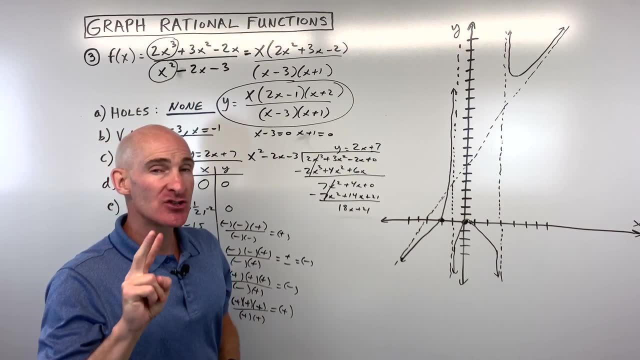 Maxes or mints. So good job on this one. This one was a slant asymptote, remember, because the degree in the numerator was one higher than the highest power term in the denominator. Let's take a look at two more examples. 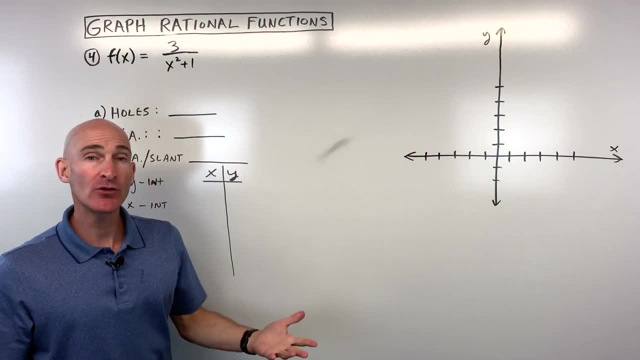 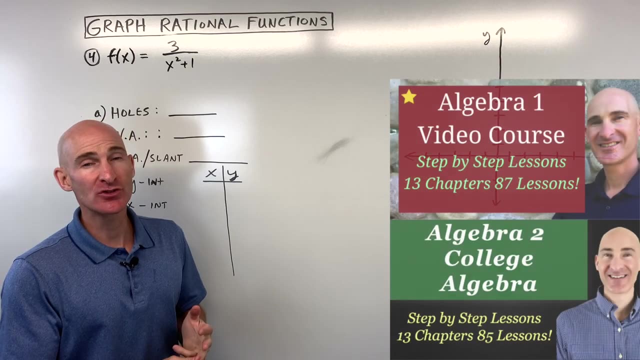 Okay, before we dive into these last two examples, if you like the way that I explain things and you want to go deeper with your math learning with me, check out my Algebra 1 and my Algebra 2 slash college algebra video courses for sale. 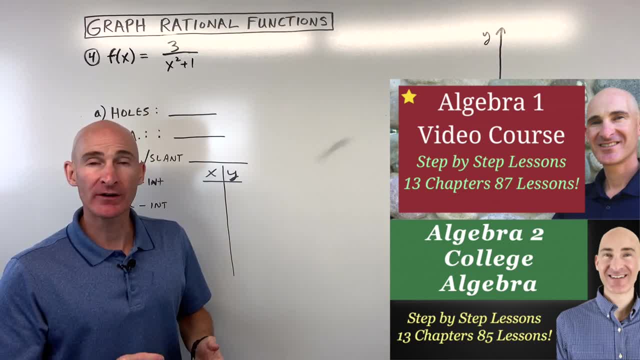 I take you step by step through a typical Algebra 1 or college algebra curriculum and I'll put links in the description below. Also, if you just want to support the videos that I'm putting up here on my Myers Math Tutoring YouTube channel: 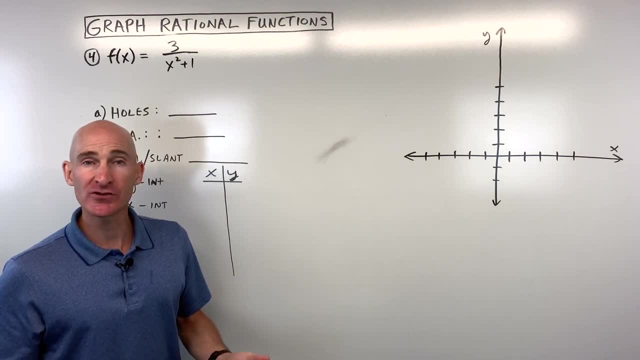 consider joining as a channel member. So for a few dollars a month you can support the videos that I'm putting up here and I really appreciate that. I see every member that comes through with the channel name or the name of your YouTube handle. 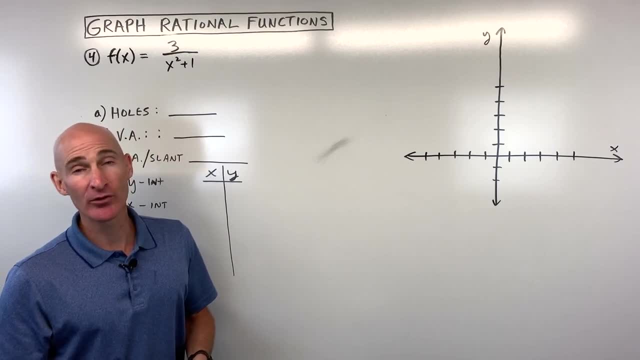 and I can see that you're a member of the channel and I really appreciate that. And then, lastly, if you just want to purchase one of my fun math t-shirts, you'll see below the video. I've got some links to my Teespring store. 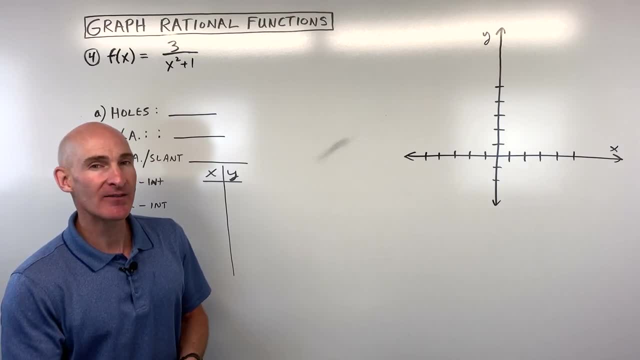 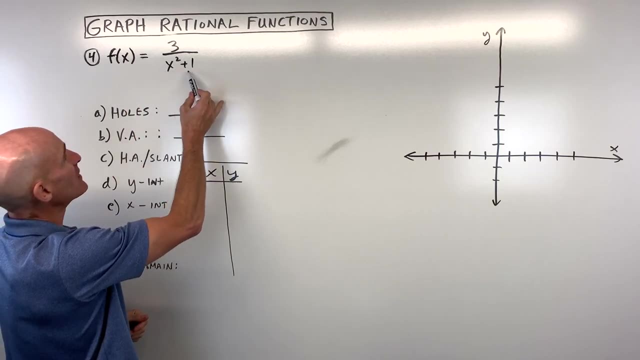 so you can purchase one of those t-shirts if you want to just kind of have some fun with my channel here. So let's dive into number four and number five. So for number four we've got: f of x is equal to 3 over x squared plus 1.. 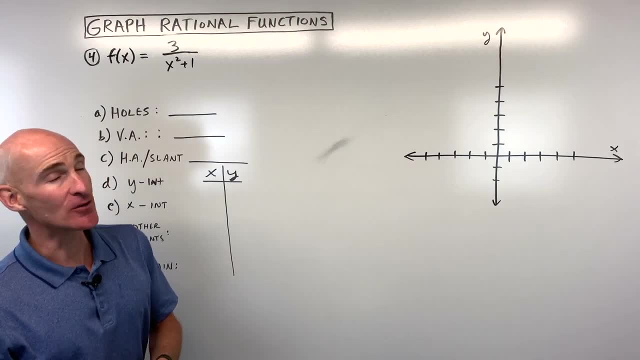 So what's our first step? First step is always to factor as much as you can, but in this case we cannot actually factor this, So, okay, we don't have to worry about that. So now, what about the wholes? Are there any factors that cancel with the numerator and the denominator? 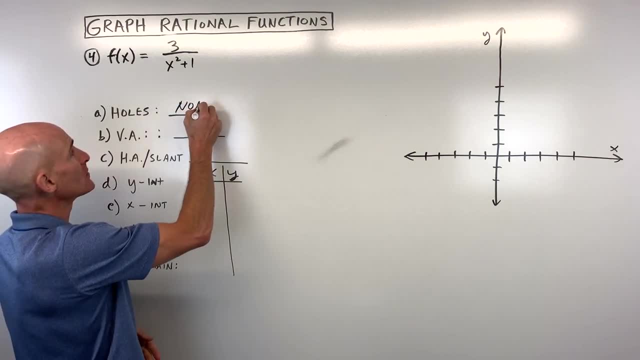 Well, in this case, no. So we're going to say: no holes here. How about vertical asymptotes? Vertical asymptotes is when we set the denominator equal to 0.. If we set the denominator equal to 0, let's just do that for a moment. 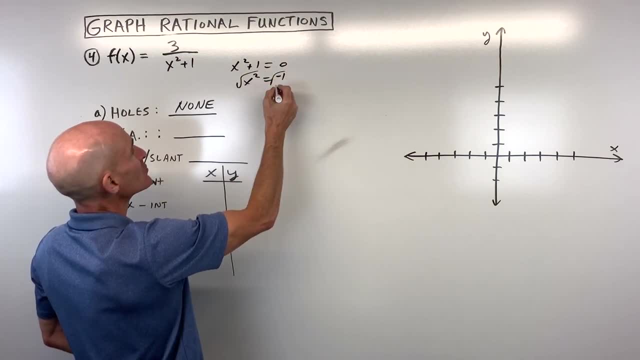 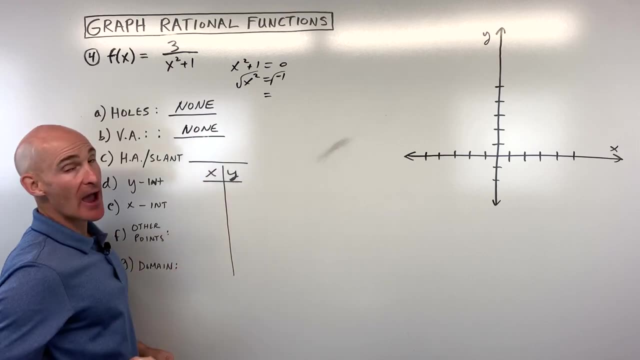 Subtract 1 from both sides. Take the square root. The square root of a negative number, you get imaginary numbers. So that tells you that there's actually no vertical asymptotes on this graph. So this is kind of a little bit different than the first three. 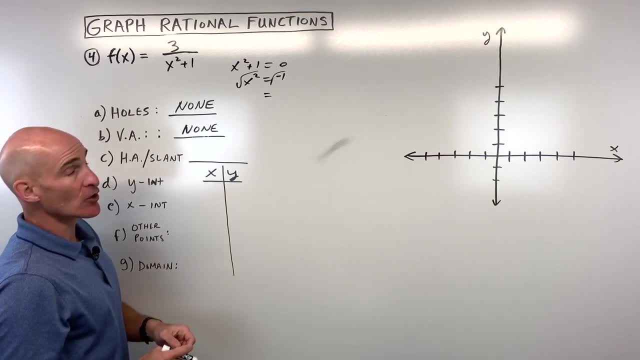 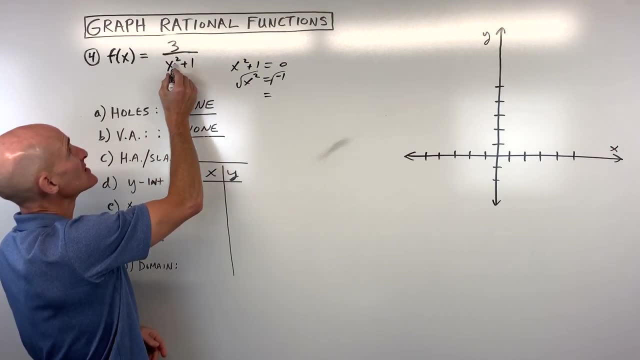 Now for letter C, a horizontal asymptote or a slant asymptote. Here's where we analyze the highest power term in the numerator and the highest power term in the denominator. So in this case, you can see, because the degree of the highest term in the denominator is higher than the numerator. 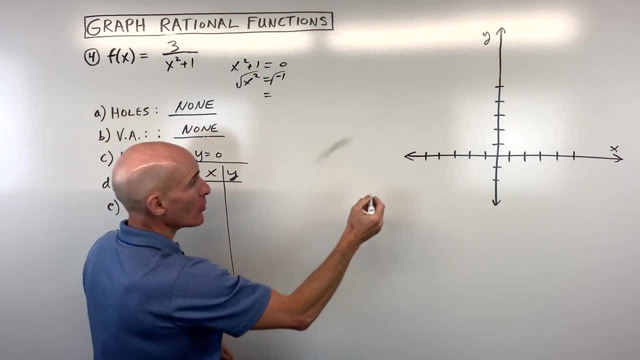 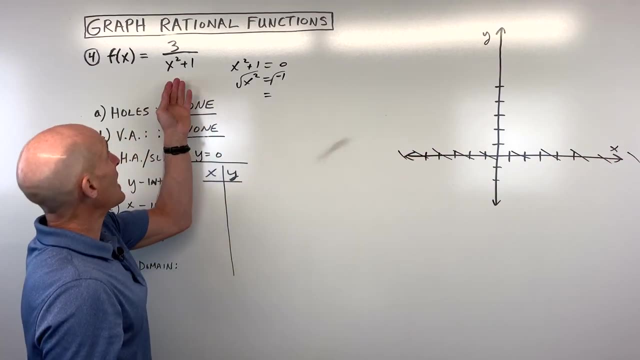 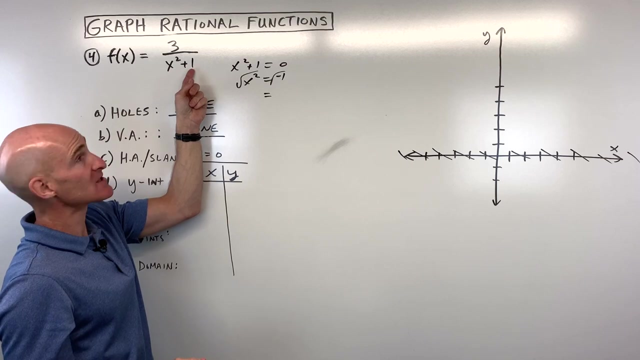 the horizontal asymptote is going to be: y equals 0, which is right here on the x-axis. And again you can think about this as x gets really large, Like say, for example, if x was like 100, 100 squared is 10,000, plus 1 is 10,001,. what's 3 divided by 10,001?? 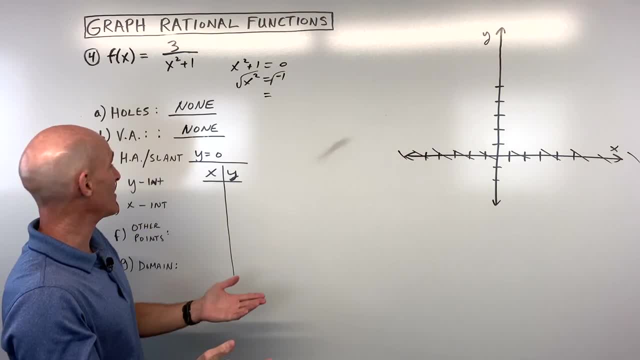 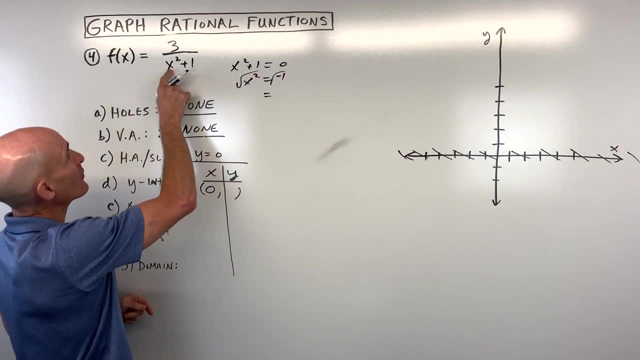 It's like .00, you know it's approaching 0, basically right. So now for letter D, the y-intercept. So to find the y-intercept, we set x equal to 0. And if we do that, we're going to get 3 over 1, which is 3.. 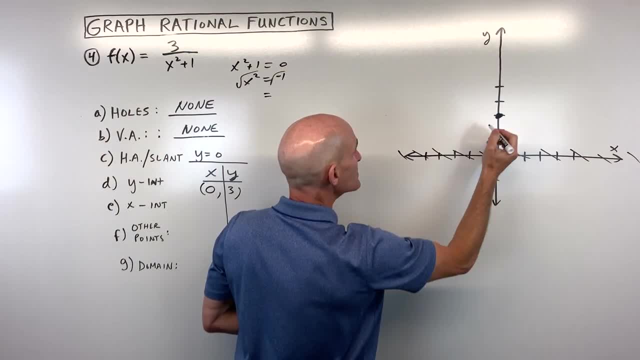 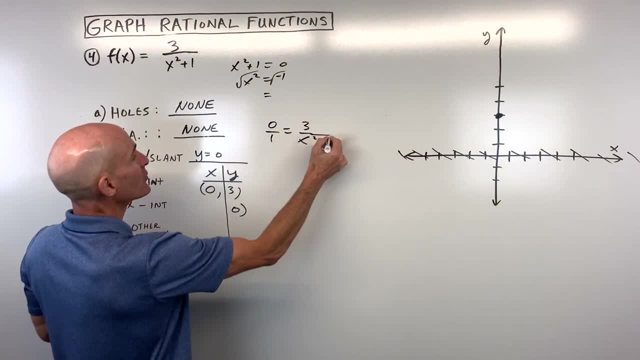 That's like 0 over 1, and if we cross-multiply here we get: 3 times 1 is 3, is equal to 0.. 3 times 1 is 3, is equal to 0. Which doesn't make sense. 3 can't equal 0.. 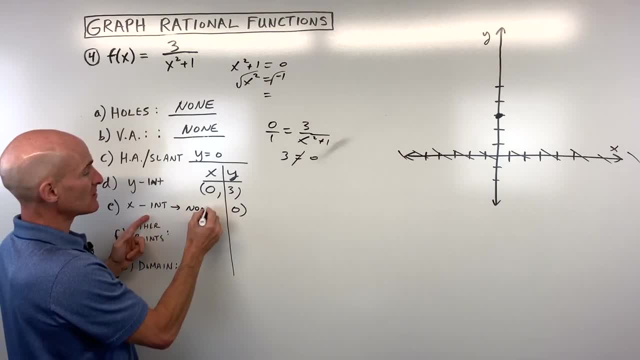 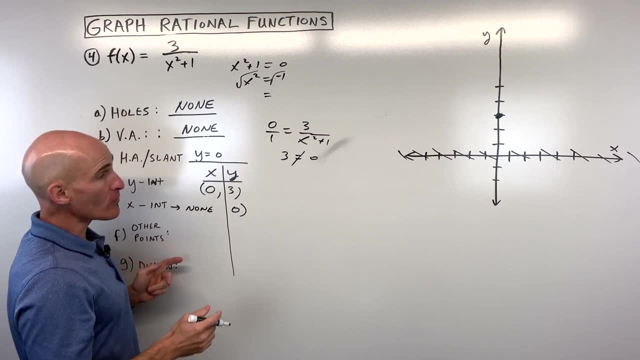 So that tells us that there's really no x-intercepts. okay, So it's not crossing the x-axis. And then let's plot some additional points. Now, normally I'll pick some points on either side of the vertical asymptote, but there's not a vertical asymptote. 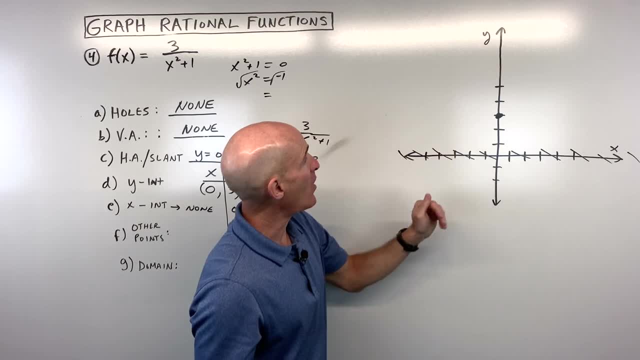 So let's just pick some points on. you know, on either side of this directly and bread lending side, side of this y-axis, Let's just do. let's say, for example, a negative 3 and positive 3.. So if I put 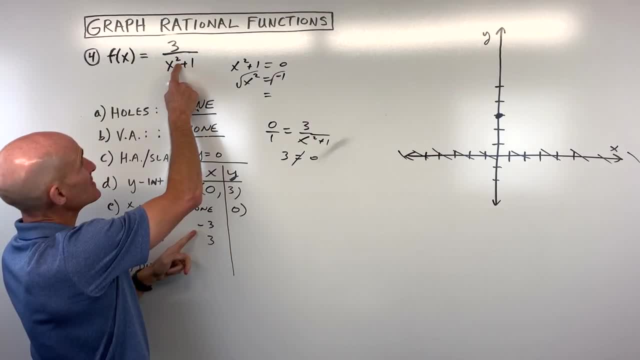 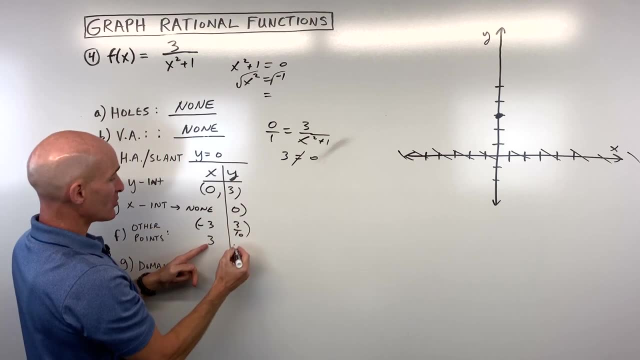 in negative 3, I get negative 3. squared is 9 plus 1 is 10, 3 over 10.. And if I plug in positive 3, I also get 3 tenths. So that's interesting. So negative 3, 3 tenths is right about here. 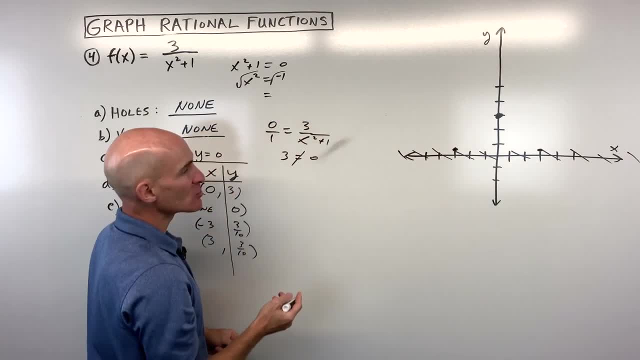 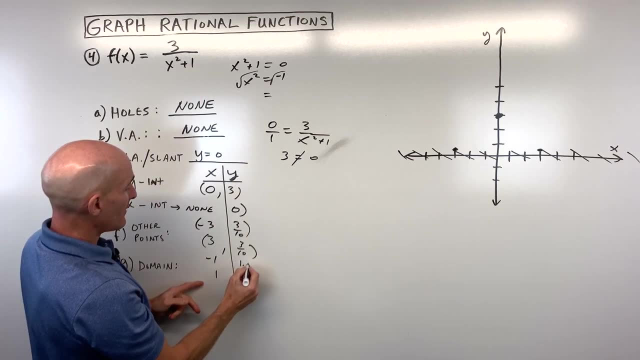 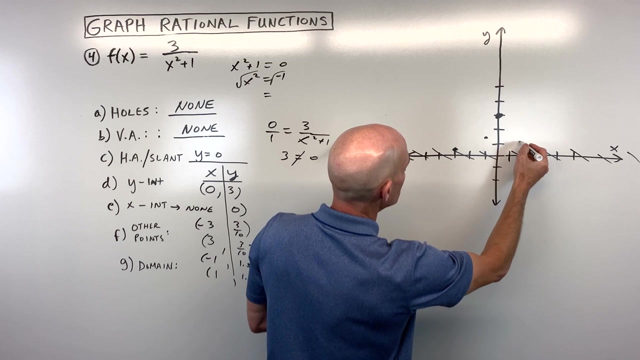 and positive 3, 3 tenths is right about here. I can plot some additional points as well, Like maybe let's plot a negative 1 and 1.. That would give us 1.5 and 1.5.. So that's going to be right about here and right about here. So you can see, this graph is basically. 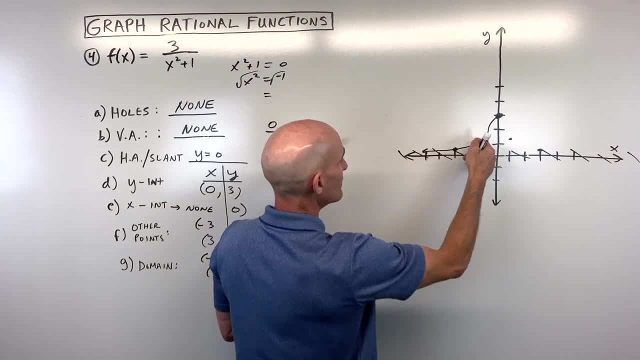 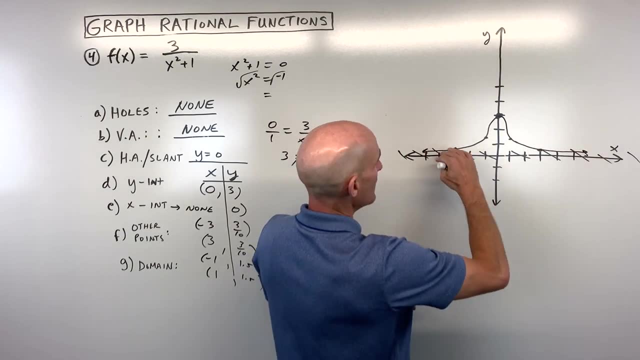 it's going like this, where it's approaching the x-axis as you go to the left. It's approaching the x-axis as you go to the right And it's like a symmetric: If you fold over the y-axis, it's going to match the y-axis, And if you fold over the y-axis, it's going to match the. 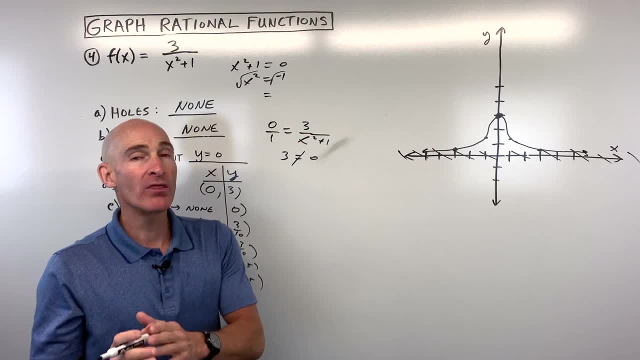 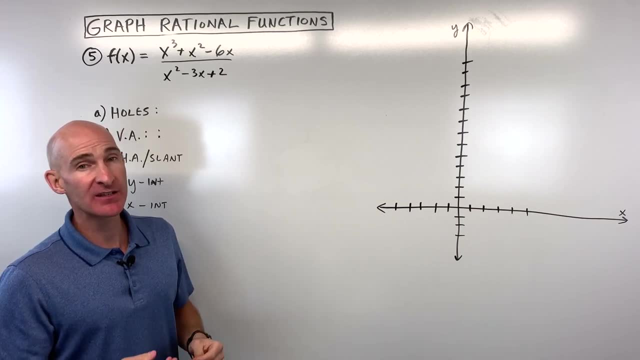 y-axis, It's going to match to itself. So this is a little bit different graph. Let's take a look at one last example. Okay, let's dive into example number five, And if you want more practice with these problems, I'll put a link at the end of this video. I'll indicate where you can click. 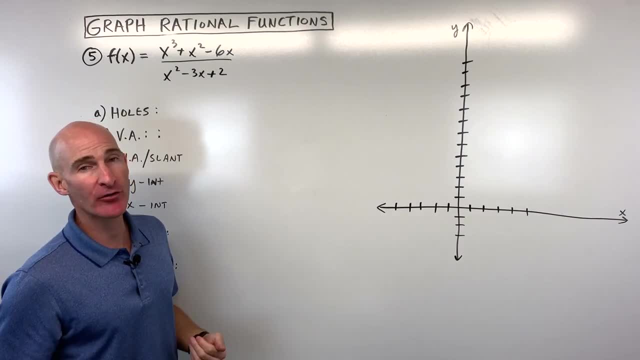 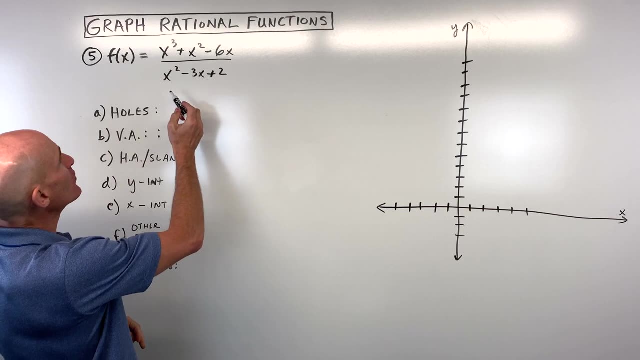 to see some other video that I did previously talking about how to graph these rational functions. But for number five, how do we graph this one? Well, this one, we notice that we need to factor it first as much as we can. So I notice I can factor out an x as the greatest common. 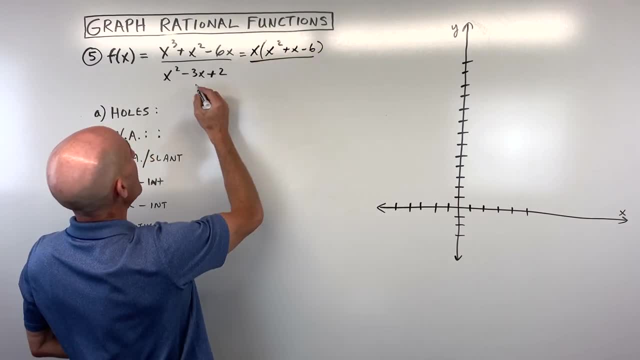 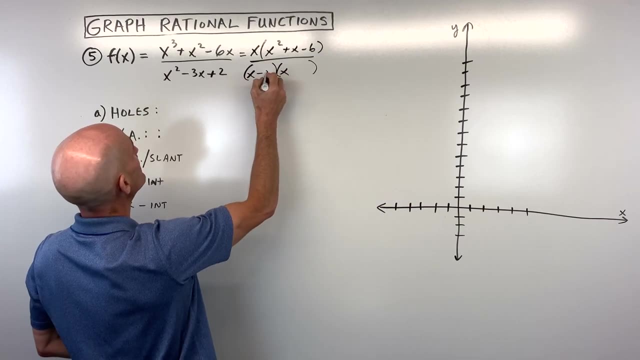 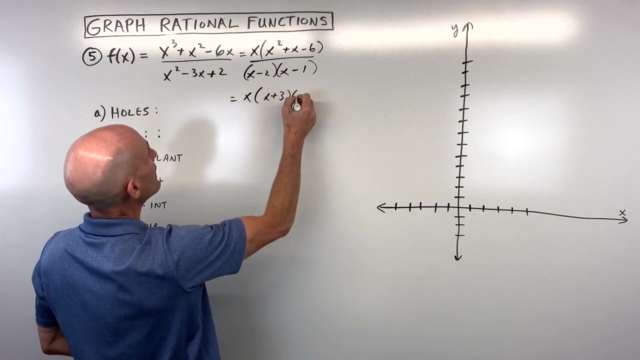 factor in the numerator And the denominator looks like we can factor into two binomials What multiplies to two but adds to negative three. that's going to be negative two and negative one, And it looks like I can factor this numerator a little bit further: x plus three, x minus two. 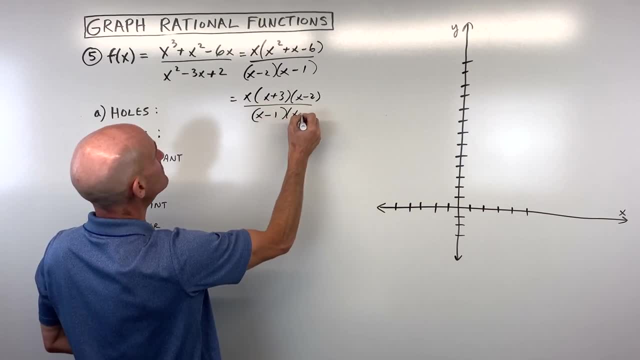 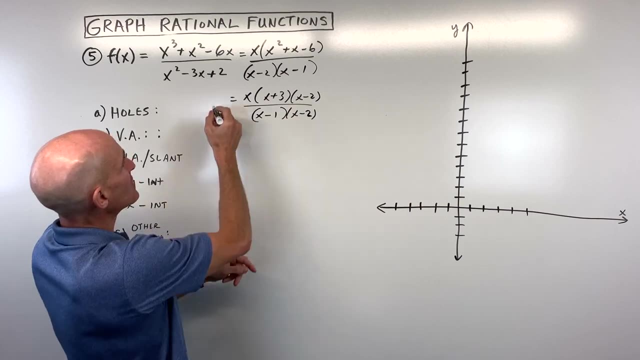 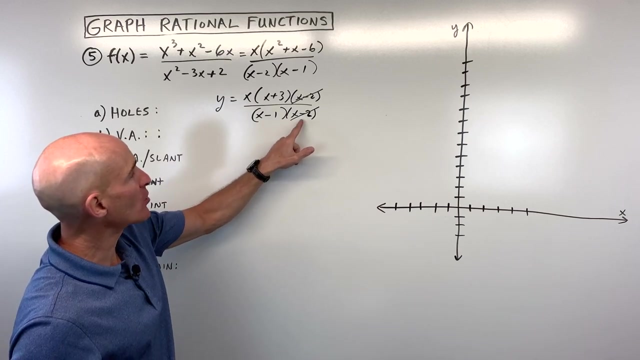 over x minus one, x minus two. I notice I just flip these And so notice here that there's a factor in the numerator that cancels with the denominator. So I can factor in the numerator so that tells us that there's going to be a hole in our graph right And that x coordinate of the 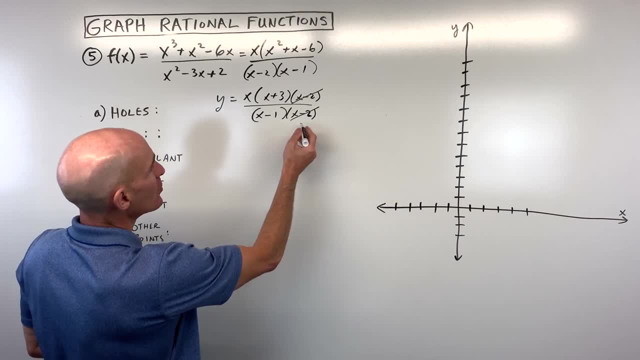 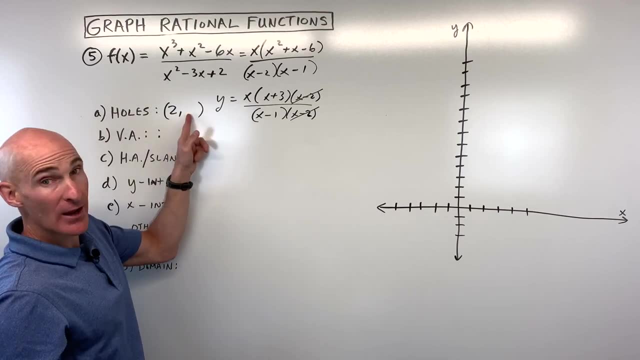 hole if we set this equal to zero. x minus two equals zero. x is equal to two. So we're going to have a hole at when x is equal to two. Now how do we find the y coordinate? We take that two and. 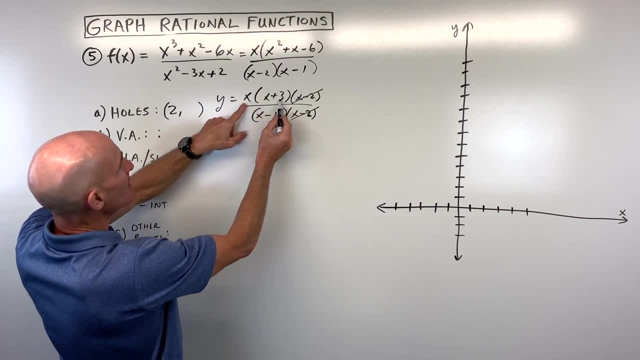 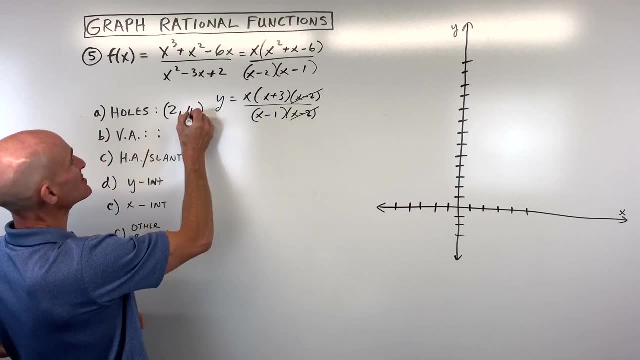 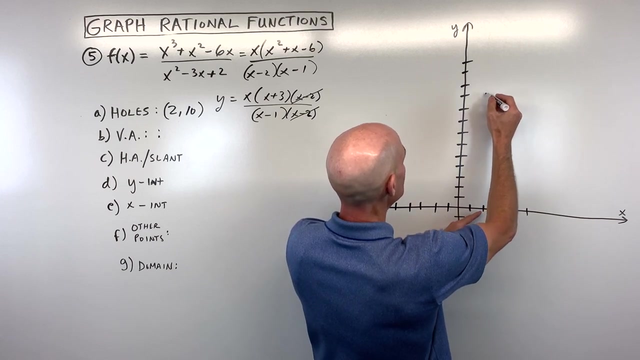 we plug it back in. So that's going to be: let's see, two times five is 10 over two minus one, which is one, So that comes out to 10 over one, which is 10.. So let's see on our graph here: two, 10, that's going to be one, two, three, four, five, six, seven, eight, nine, 10,. 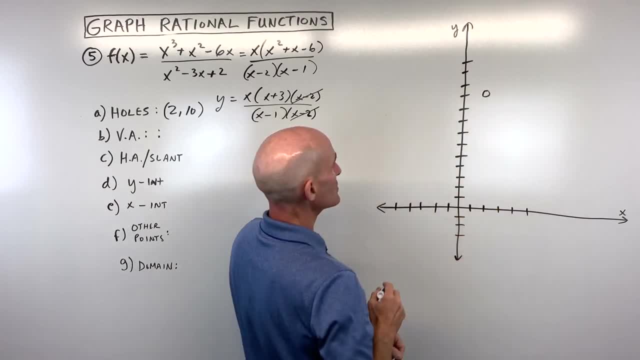 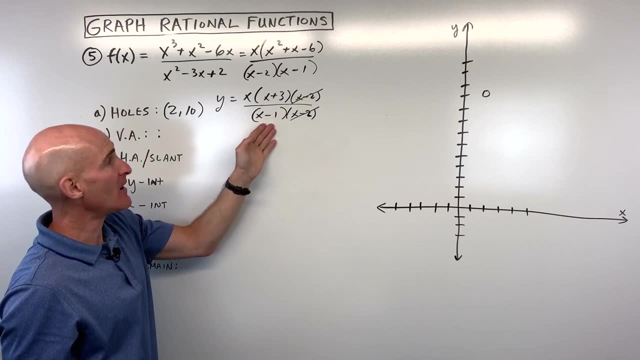 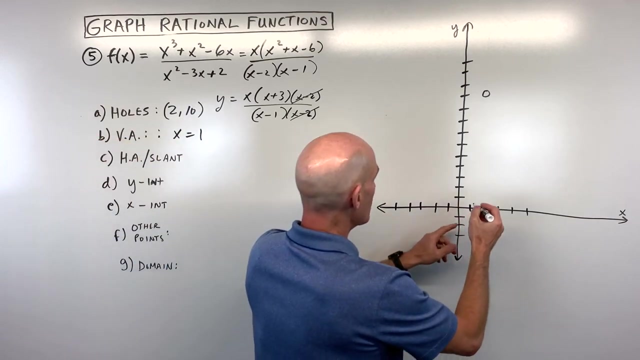 right about here. okay, is our hole. Now for the vertical asymptotes. we want to set the denominator equal to zero, because we can't divide by zero. that's undefined. So if I set this equal to zero, that means that x equals one- would be our vertical asymptote. So that's going to be right here. 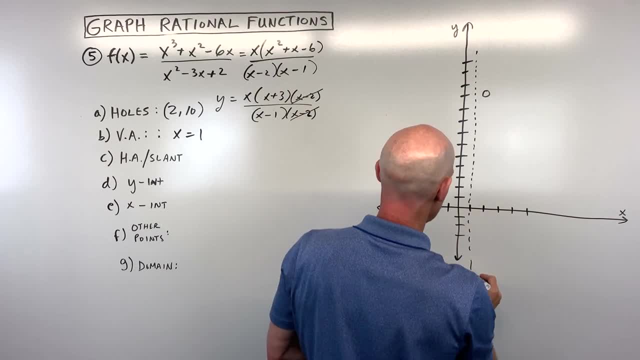 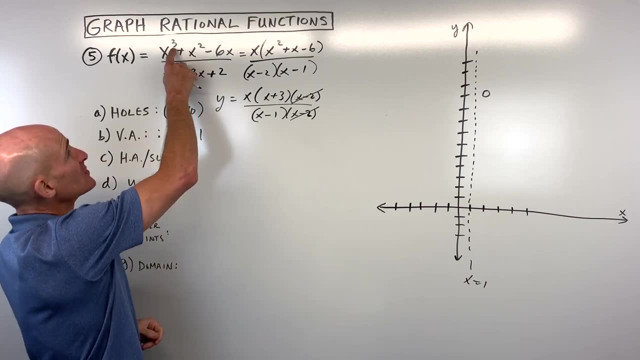 Let's draw this as a dashed or dotted line right through. x equals one. And then for our horizontal or slant asymptote, which one do you think it is Well notice that the degree in the numerator is one higher than the highest power term in. 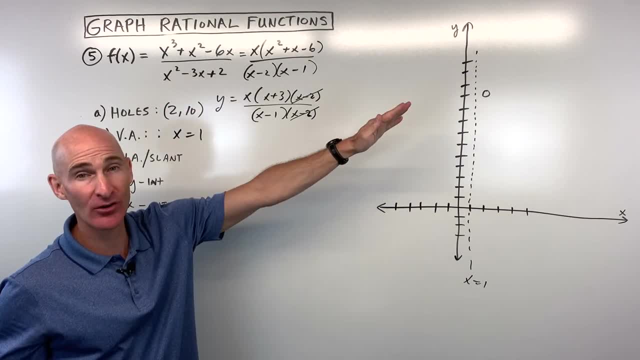 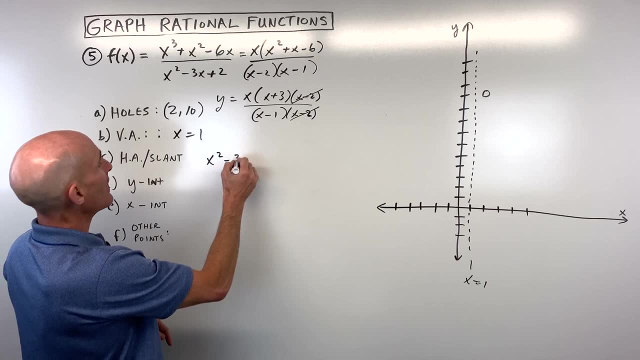 the denominator That tells us we're going to have a slant or a diagonal asymptote, And the way that you find the equation of that asymptote is to do some long division. So we're going to figure out: how many times does x squared minus three? x plus two go into the numerator x cubed. 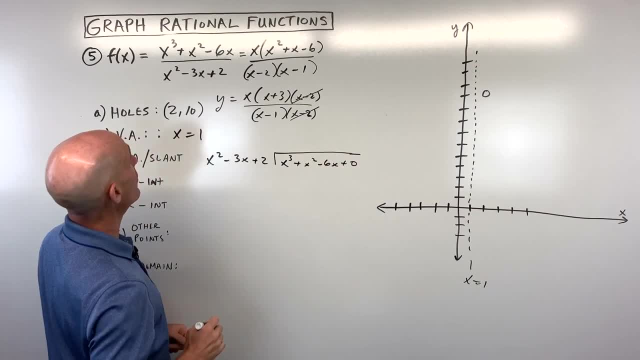 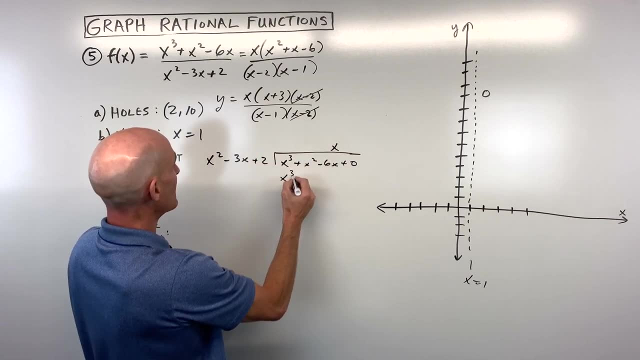 plus x squared minus six x. So this is the WhatsApp slant eight. so the square root of the square root of x plus zero equals x squared times eight. x plus zero. So x squared goes into x, cubed x times. if I'm going to distribute the x to all three of these, 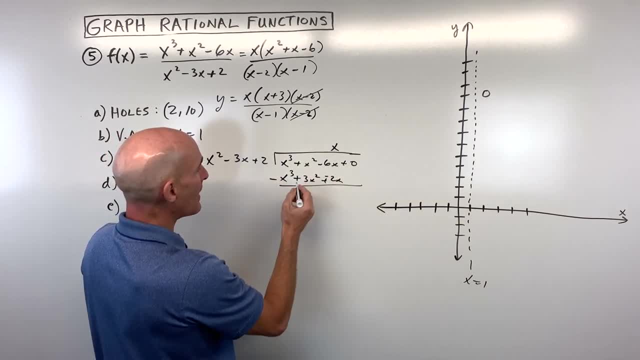 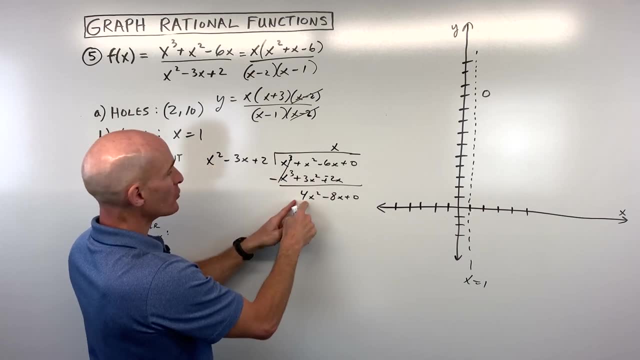 terms, that's going to give us x cubed minus three x squared plus 2x Subtract. or you can change the sign to the opposite and add So that gives us four x squared minus eight x plus zero. How many times is x squared going to four x squared? That's four times If I distribute the. 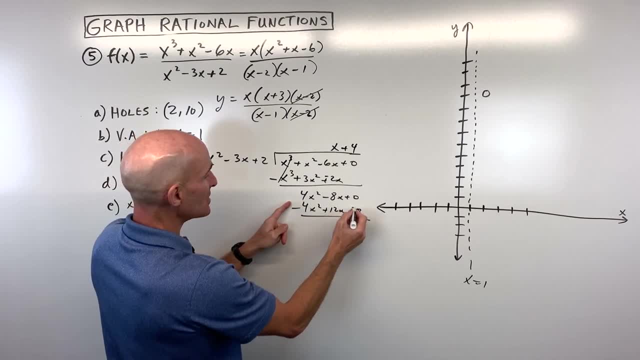 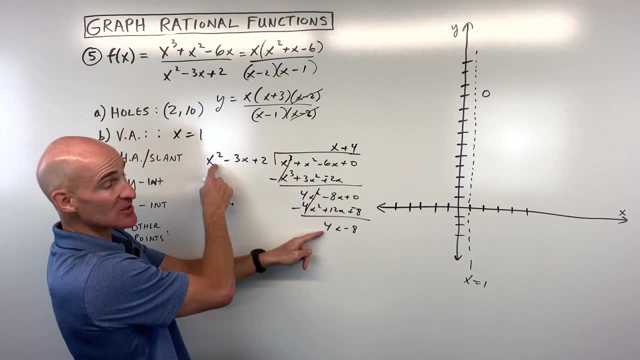 this and if I subtract, which is like changing the signs to the opposite and adding, we get 4x minus 8 and notice that this is x to the first. this is x squared. Normally what we do is we put our remainder over our divisor right when we do our long division. 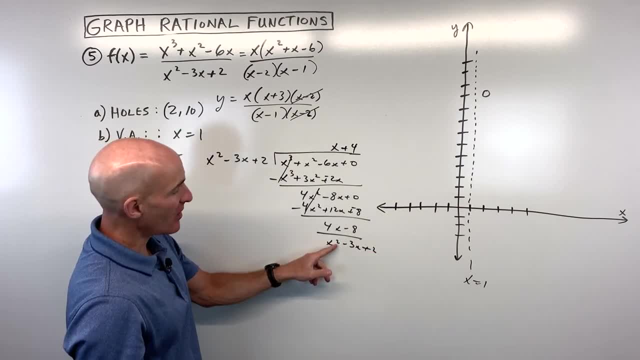 but what happens is see as x gets larger and larger, this whole fraction is going to go to zero, because the degree in the numerator is higher than the degree in the degree in the denominator is higher than the degree in the numerator, so this whole thing goes to zero. 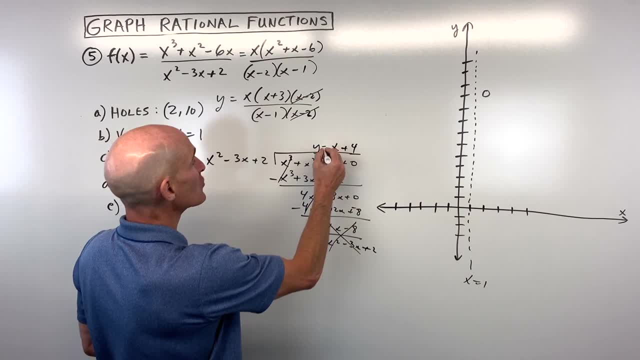 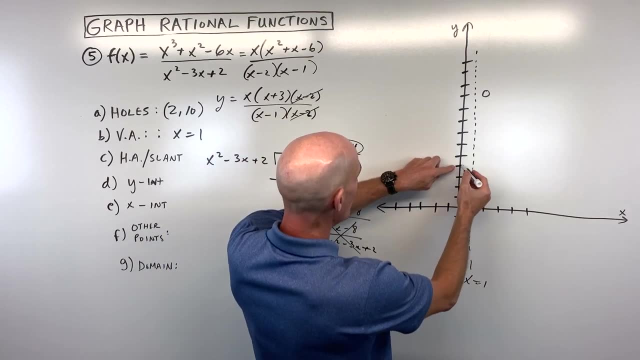 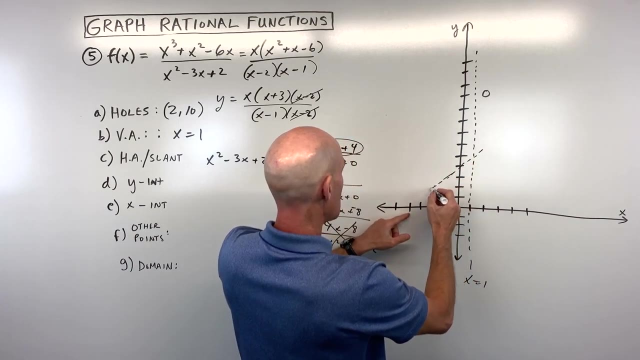 that's why I say we don't have to worry about the remainder. our slant asymptote is just going to be: the line y equals x plus 4.. So let's even graph that. on our graph we have a y intercept of 4 and a slope of 1, so it's going to go like this. try to be accurate here as much as I can. 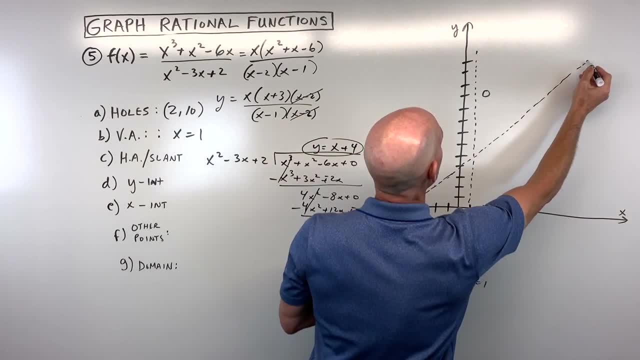 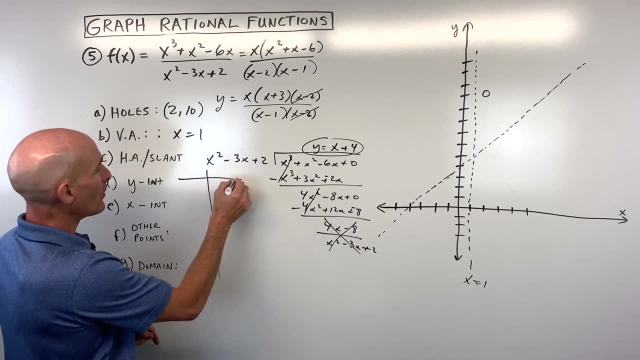 something like this: Okay, there's our slant asymptote. now let's analyze our y intercept and our x intercepts. what I like to do is make a table and you set the opposite variable to zero. so if I want the y intercept, I put zero in for x, if I put zero. 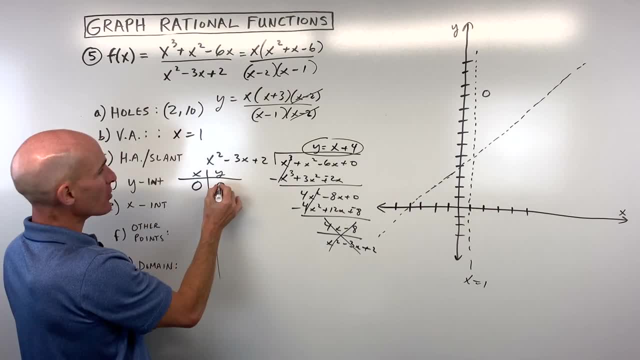 in for x. you can see I'm going to get zero over two, which is zero. so that means it's going to go right through our origin here at zero zero. if I want to find the x intercept, I set the y equal to zero. now the only way that y is going to equal zero here is if the numerator's factors are zero. 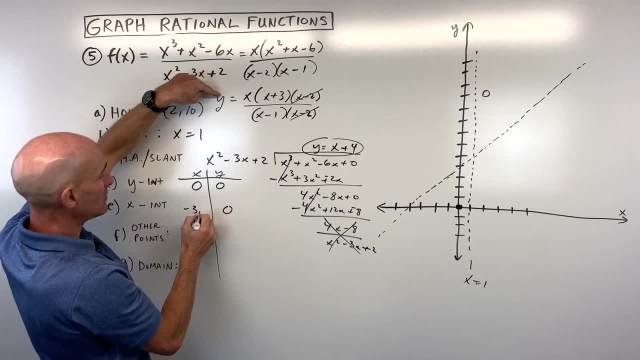 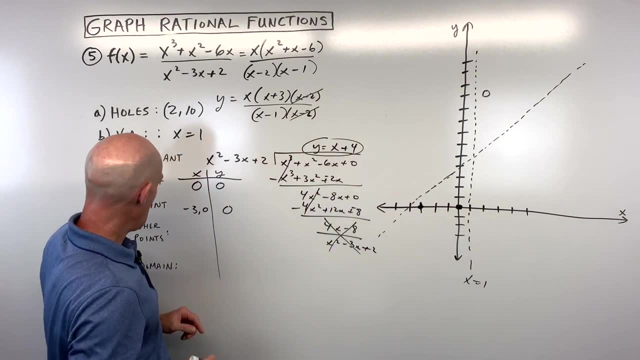 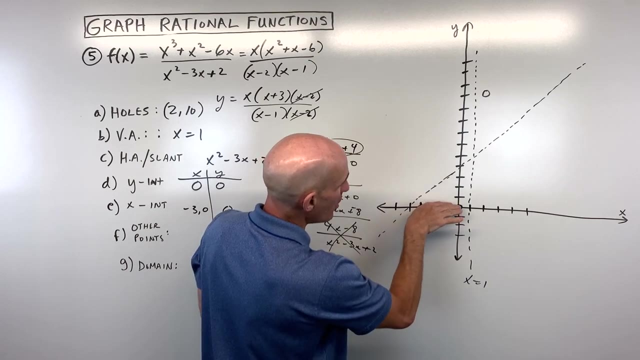 so that would occur at zero and negative three. so that means it's going to cross at zero and negative three. Okay, right here, and then let's plot some additional points. now the key points are the points on either side of the vertical asymptote, because, remember, it's like a brick wall. it either has to go down. 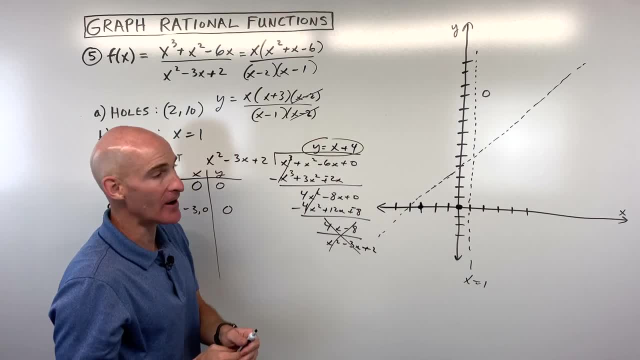 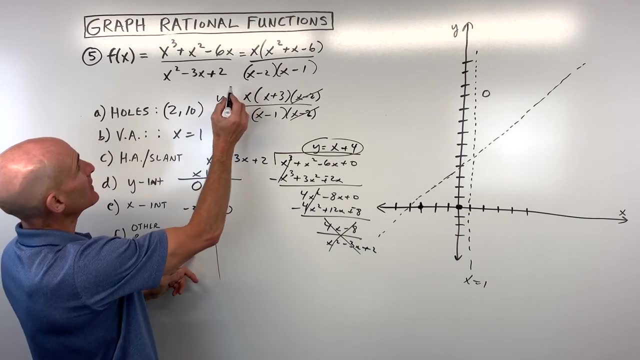 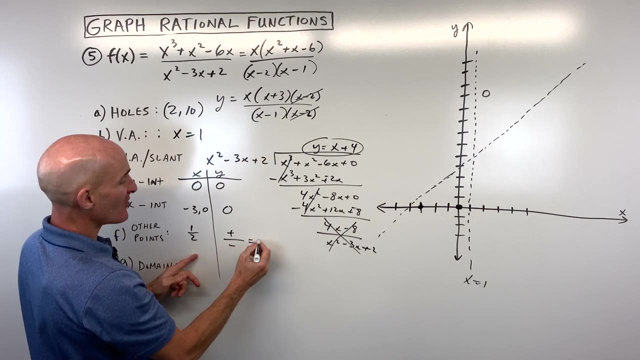 to negative infinity up through positive infinity can't go through the brick wall, right? so let's maybe plot a half. so if we put a half in what happens, we get a positive, positive which is going to give us a positive when you multiply over a negative. a positive divided by negative is a 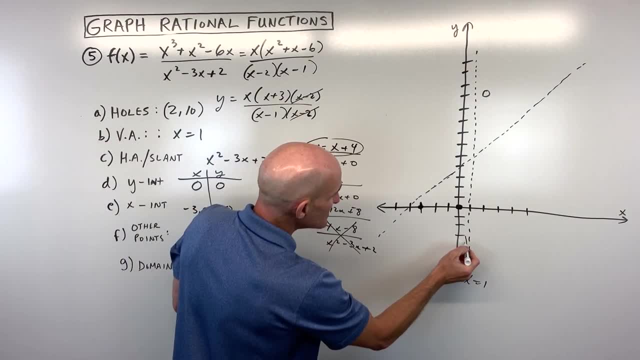 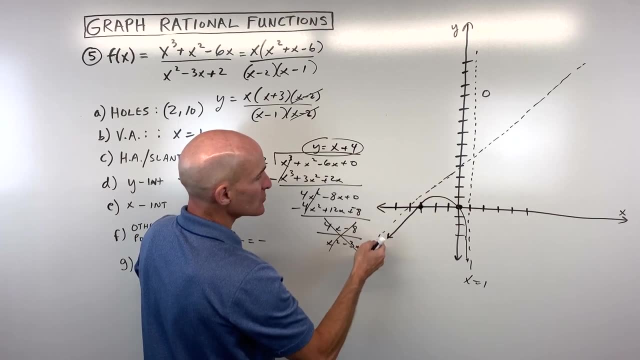 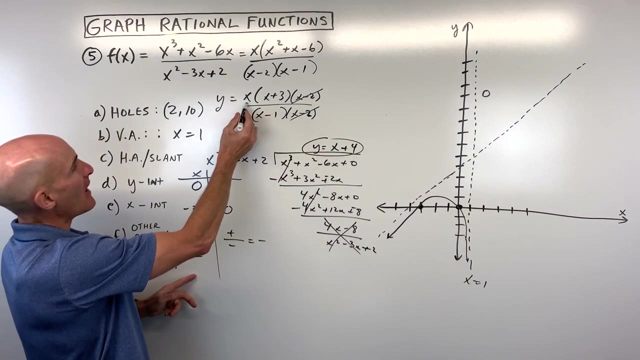 negative. so that tells us it's going to go down like this. so we can see what's happening here: the graph's going like this and like this, approaching that slant asymptote getting closer and closer. now if we pick a point on this side, let's say, for example, like two, that's going to give us a positive. 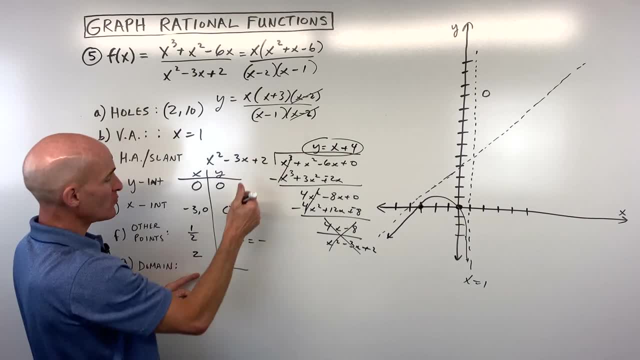 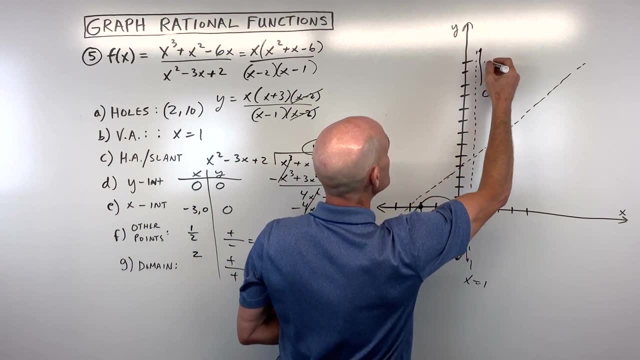 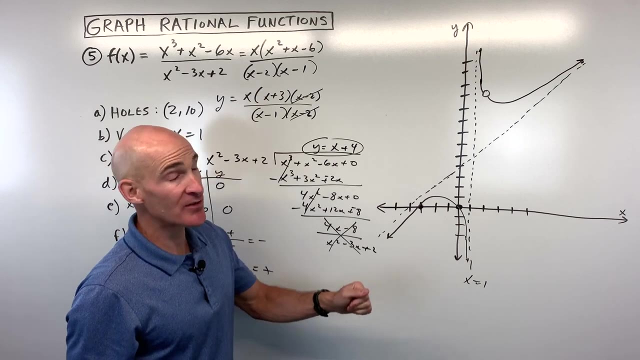 positive, which is a positive, over two minus one, which is positive one, that's a positive. a positive divided by positive is a positive. so from this side, it tells us this graph's going to go up towards positive infinity. Now, this graph's going to go something like this: okay, now again. we talked about this in a previous. 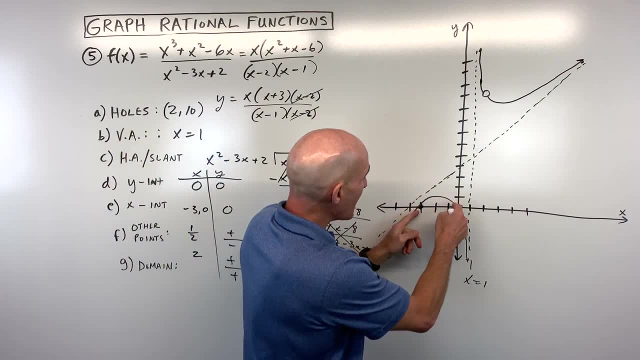 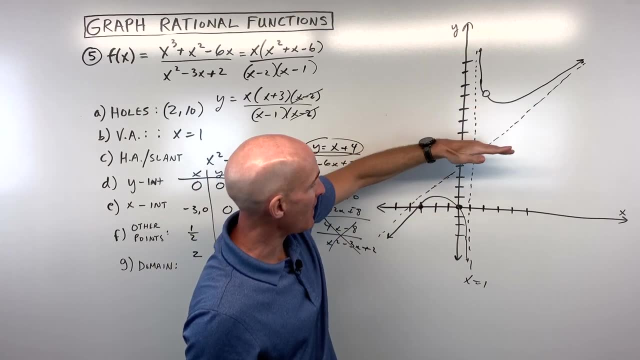 example, we don't know exactly where this graph is bending without using calculus. we have to find out where the slope of the tangent line is equal to zero, to find these extram of these maximums and minimums. but for this video, for this what we're doing here, we're just getting a basic sketch. we've 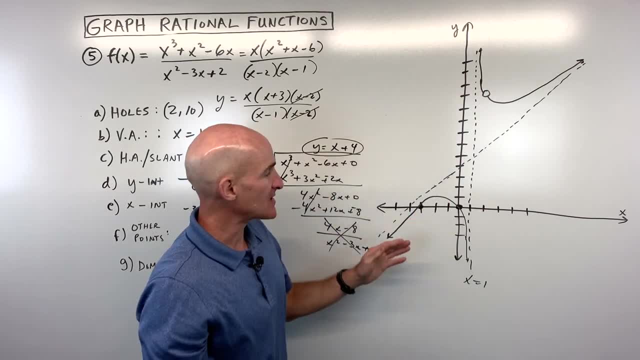 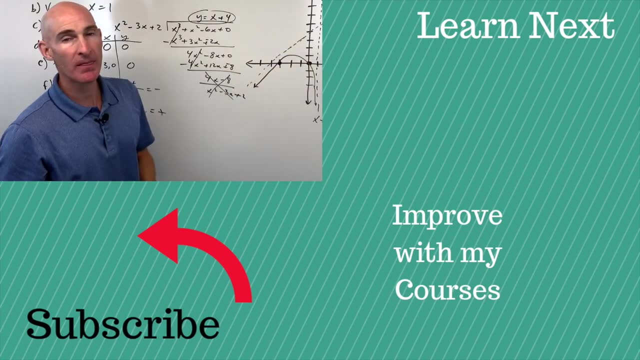 got our intercepts, we've got our asymptotes, we've got our holes, we've got some, you know, sign analysis to tell us if the graph's going up or down To the right or down to the right up. you know, with the asymptotes, where it's approaching, etc. 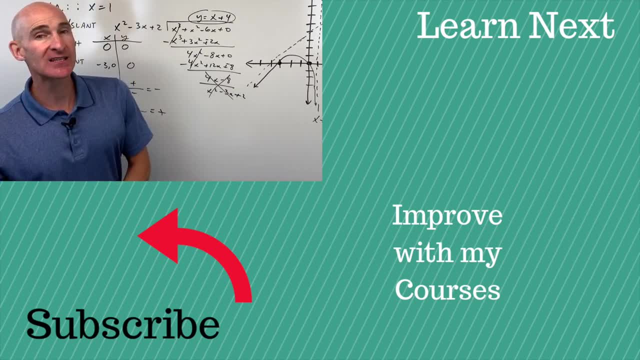 So great job. I hope you picked up some good pointers in this lesson, but if you want more practice, follow me over to that video right there where we dive into some more examples graphing rational functions. I'll see you in that video.